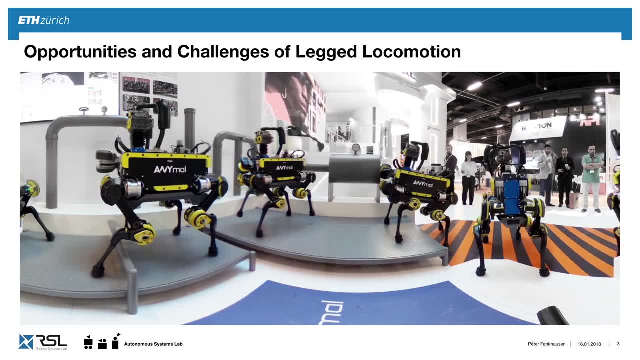 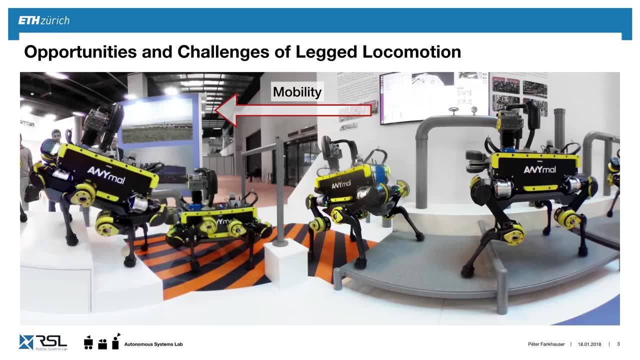 even go up and down stairs. In my work, I want to focus on the mobility of legged robots in rough terrain. There are several key constraints that we have to take into account. The robot has to make contact with its feet on an intermittent basis. It has to choose stable footholds in order to 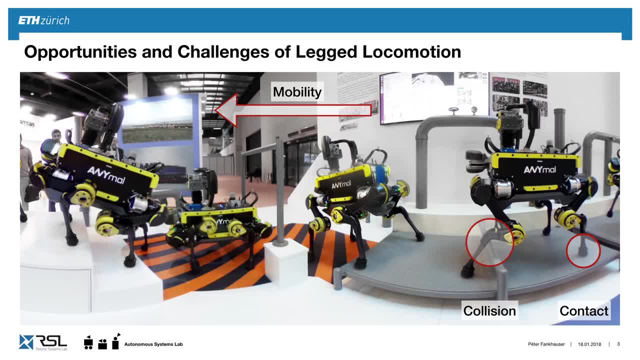 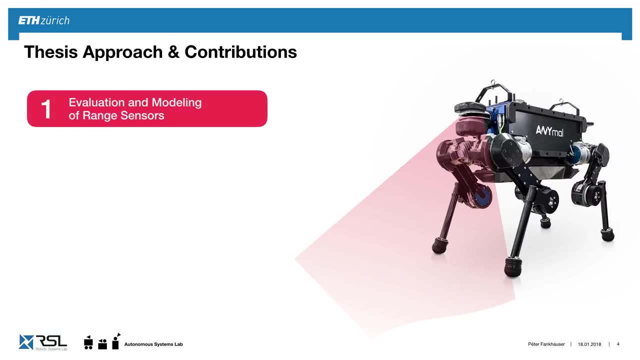 locomote, It has to make sure it doesn't collide with the environment. Then it has to all the time keep stability and make sure it doesn't collide with itself and keep joints and tortuous mutations. I'm going to structure my work in five parts. I'm going to start with the evaluation and 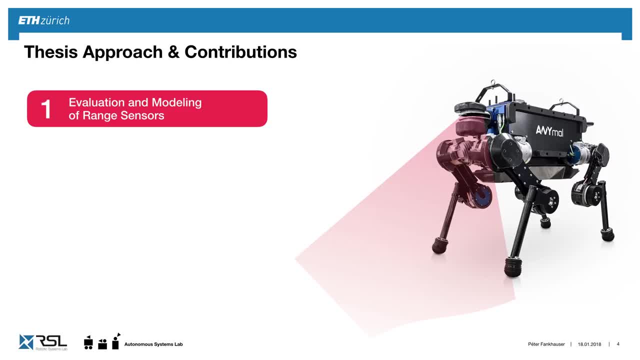 modeling of one center, so the robot has to perceive first its environment in order to understand it When it takes these measurements. I'm going to look at terrain mapping, where the robot takes sense out of this data and creates a map that is understandable to the 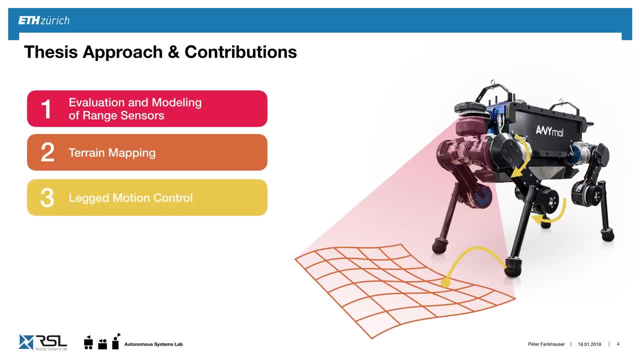 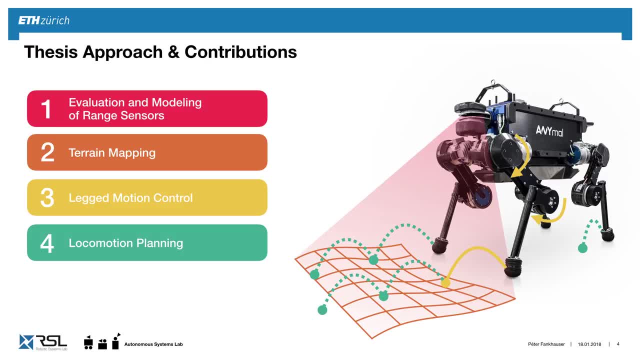 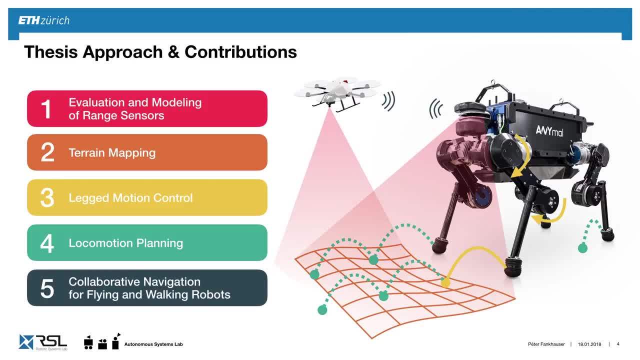 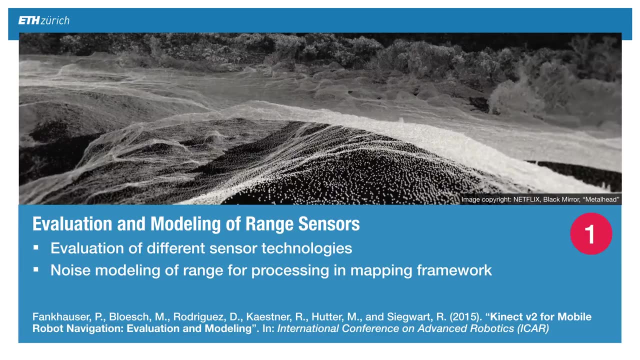 And finally, I'm going to broaden the context and look at collaborative navigation for flying in the wheeled vehicle to improve their navigation skills. I'm going to start up with the evaluation and modeling of one sensors, And here we're going to look at different technologies. My goal is to model and understand the errors. 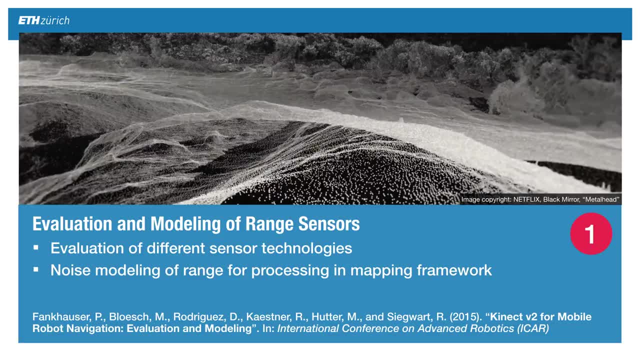 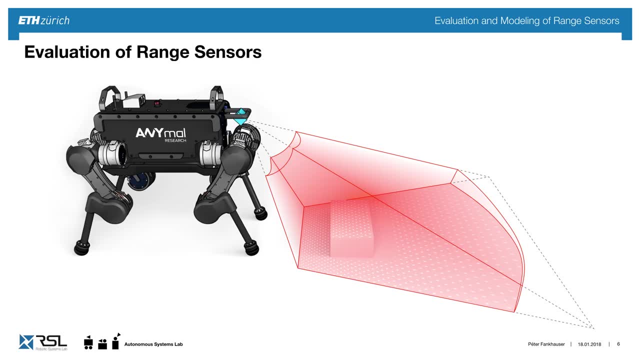 and the noise that we get from the sensors, because understanding the area means we can create high quality maps from this data. So, looking at the performance criteria, here we have the robot with a sensor in front of it, and important criteria are measurements such as minimum and maximum range. 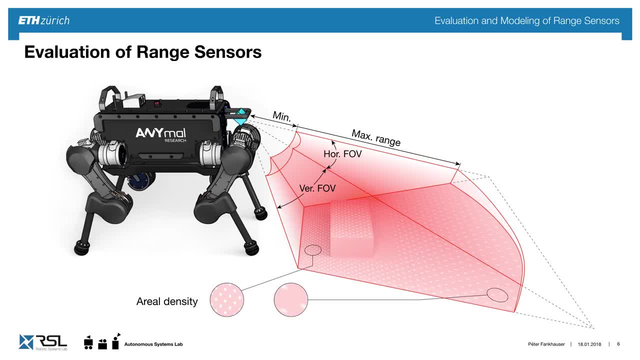 horizontal, vertical, field of view, but also, importantly, the density, the number of points that we get out per measurement. We have to make sure the sensor works in sunlight and, like I mentioned important factors, what is the resulting error when taking these measurements? 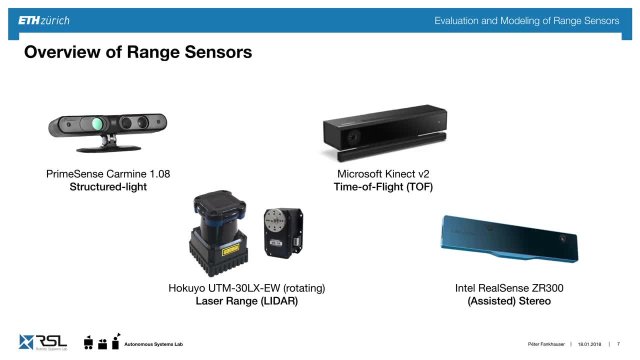 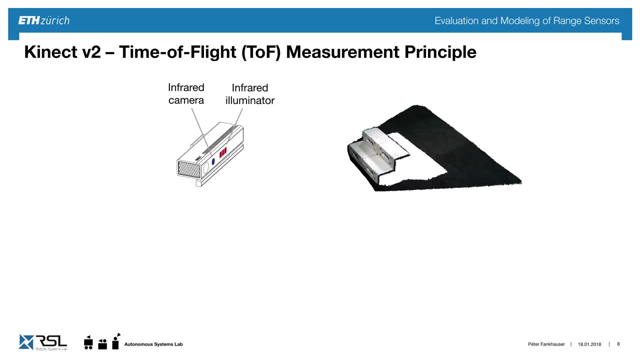 I have evaluated four different sensor technologies, mainly structured light, laser range or LIDAR, time of flight cameras and assisted stereo cameras. In the following I wanna focus on the noise modeling of the Kinect version two time of flight camera. This camera works by strobing an infrared light. 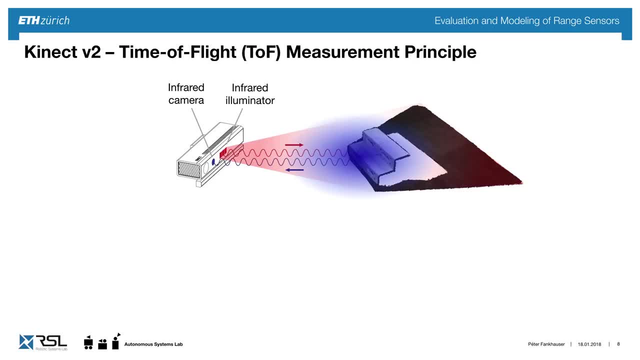 onto the scene, from which it is reflected back to a sensor. By measuring the phase difference, we can measure the time of flight that takes each ray and we can create the depth image for each pixel in the image- What I'm interested in here- shown for one ray. 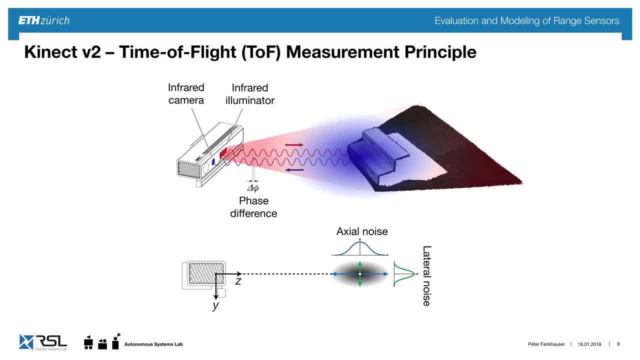 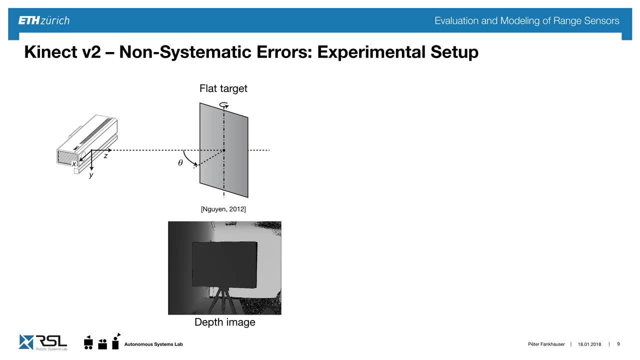 is the axial noise along the measurement ray and the lateral noise which is perpendicular to the measurement ray. To do this, we have set up an experiment where we use a target at different distances in which we can rotate, And on the left you see an image. 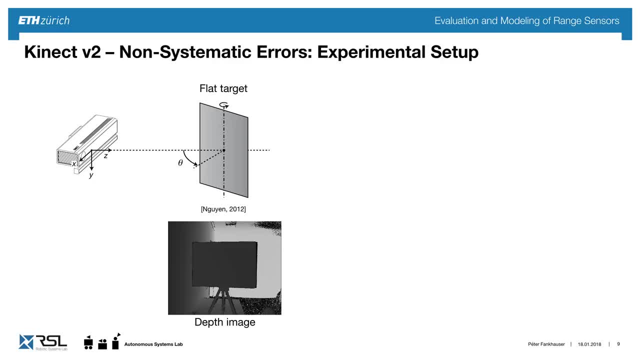 a sample image of the resulting depth image From the top view. we can use the angle theta to measure the target angle and alpha to model the some horizontal incidence angle And in this view you see how we measure the axial noise along the measurement ray. 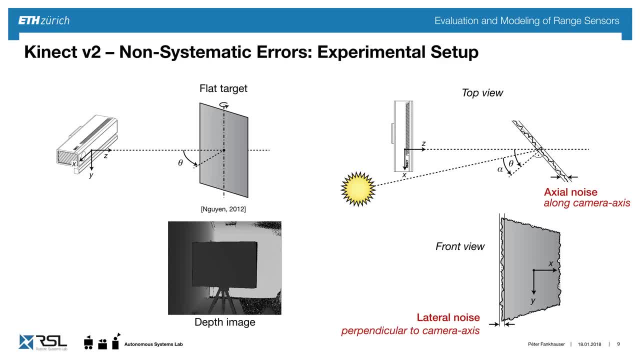 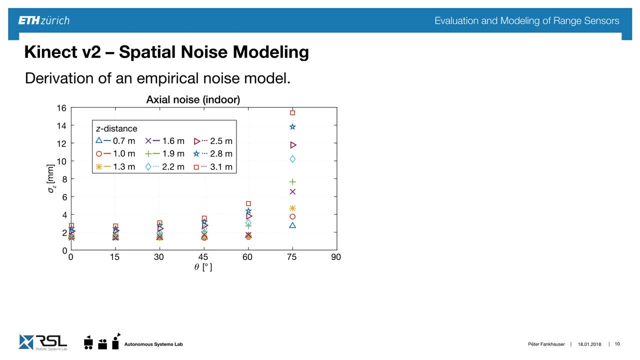 From the front view we're interested in the lateral noise. by looking how sharp can we recreate an edge of the target. By taking many measurements at different distances and angles, we get this plot Where we see how the noise increases over distance and over the target angle. 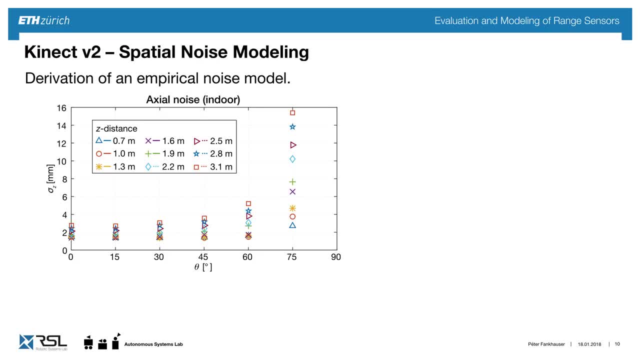 The target angle is plotted on the horizontal axis and the noise on the vertical axis, And then colors are the different ranges where we measure that. So we came up with this empirical noise model which very accurately predicts the noise at these different measurements. For the lateral noise there's no such color tendency. 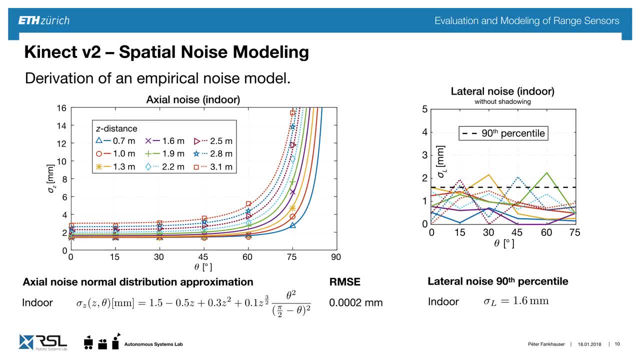 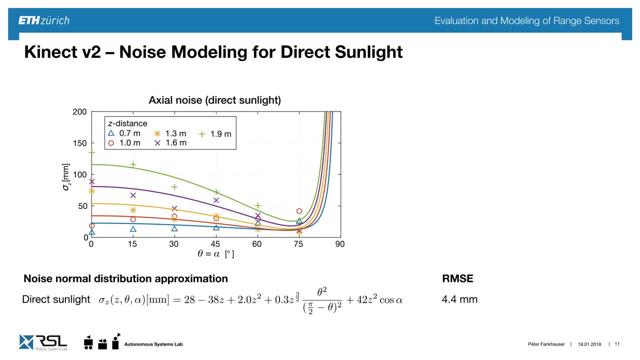 and we choose to model the noise as the 90th percentile. If we go out in sunlight, we see a different behavior, where at more direct angles of the sun we have higher noise, And we can understand this by looking at the Lambert's. 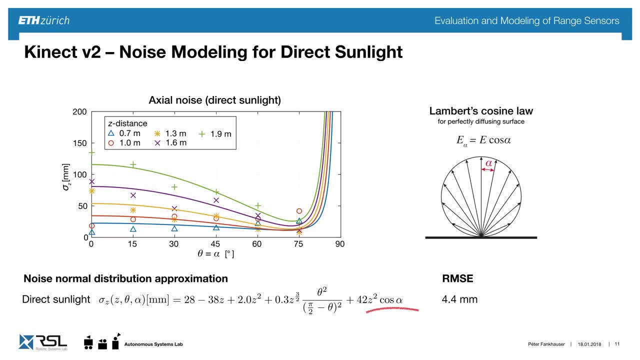 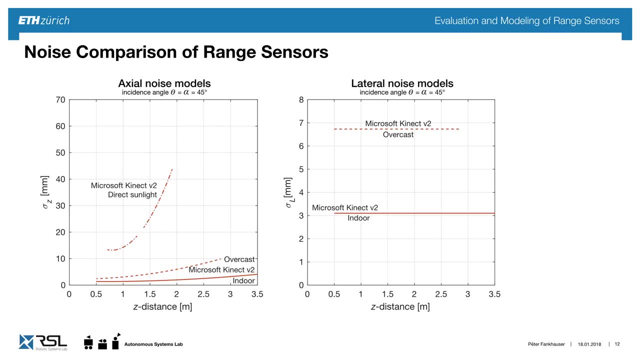 Cosine Law, which explains the light intensity as the sunlight hits the target, And we introduced this additional term depending on the sunlight angle alpha. And we can see that tomorrow. we go outdoors from indoor overcast and direct sunlight. On the left hand side we see 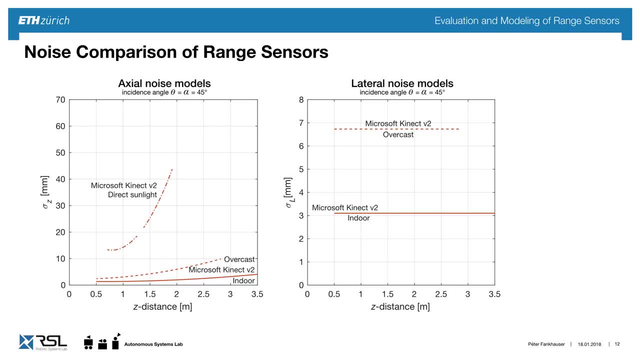 the axial noise and on the right side some of the lateral noise. And the more we go outside, the noise in sunlight is order of magnitudes bigger than indoors, And if we compare this to all the other sensors, we see a similar behavior. 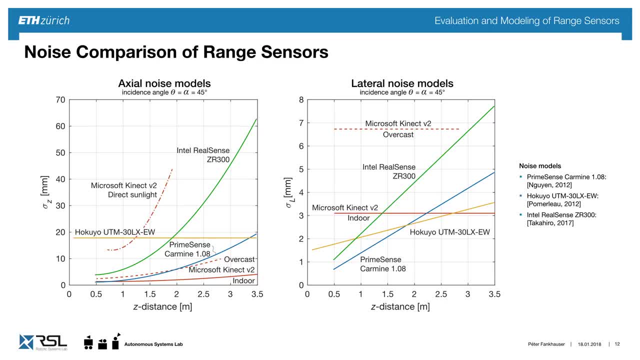 And we can say that for a range that we're interested in, with a walking robot, from one, two, three meters, the noise is in a range where it's acceptable in order to create the map that is useful, And we can also see that the noise deviates. 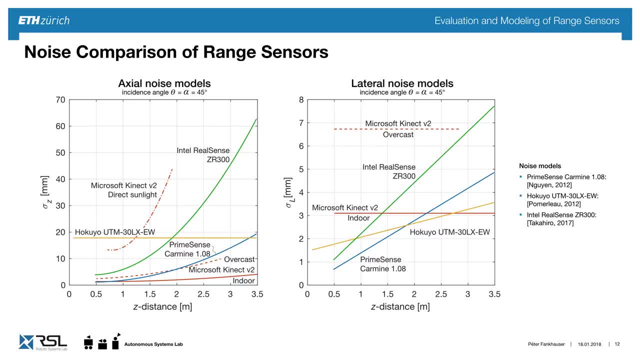 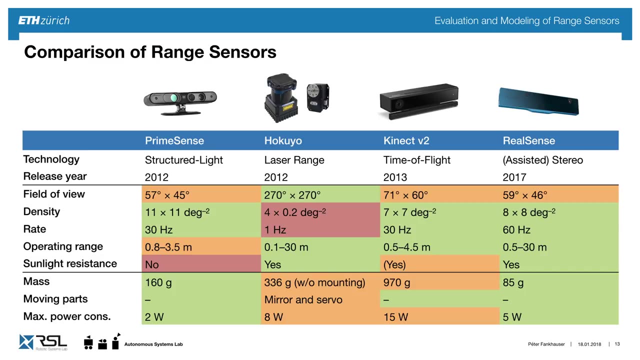 from very low to high noise at distances such that we really need to take care of this noise in order to create the best quality maps that we can get. Looking at other measurement characteristics, this table can inform us how to select a sensor for our mobile robot and our use case. 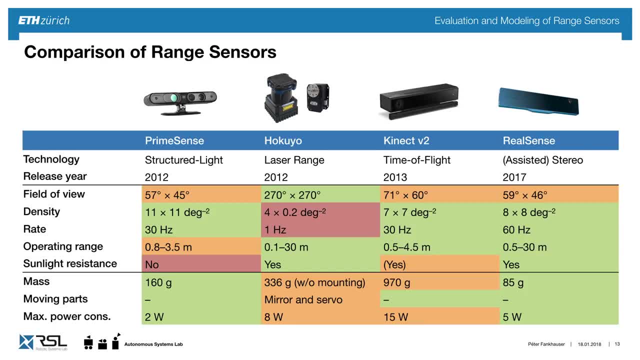 So in one example, the prime sensor, the first sensor, is really not sunlight resistant, so it could not be used outdoors. Another important characteristic is the density and the rate of these sensors, where all are good, but there's one really lacking behind. 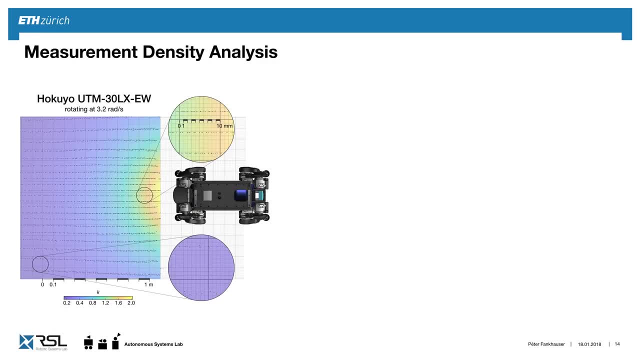 And I want to explain that in the following example. Here's a top view of the robot and you see the measuring points taken for one rotation of this LiDAR sensor. You see in the close-up, it would take two seconds to cover a one-by-one centimeter area. 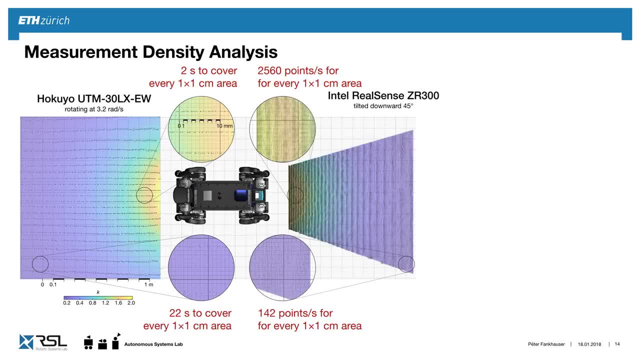 And for further weight points. it takes up to 22 seconds to cover every cell. And this is in comparison to the Intel RealSense stereo camera where we get that many points in close-up, up to 2,500 points per square centimeter. 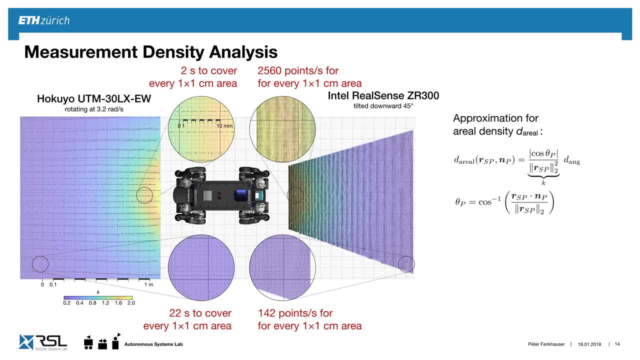 which is probably more than we need. So we can approximate this noise amount with this model, which runs depending on the surface normal and the distance from the sensor to the point. We can then use the inverse of this model to predict what is the ideal resolution. 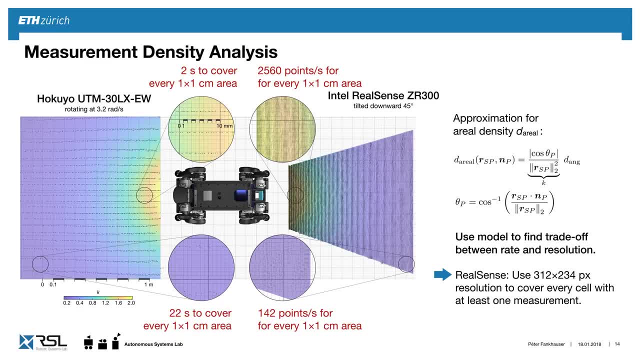 that we want to run these sensors at. So for the RealSense, in this case, we want to lower the resolution to a resolution of 312 by 234, to cover every cell at least once, with one measurement. Now that we have understand these sensors. 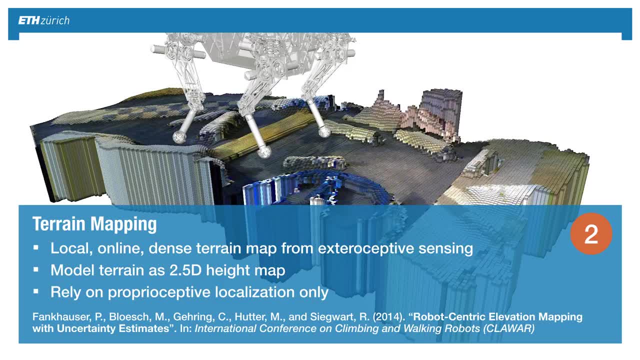 look at terrain mapping And here the goal is to locally create the map online, dense representation of the terrain from these sensors. We're going to model the terrain as a 2.5D surface map to represent the terrain And, importantly, we're going to only rely 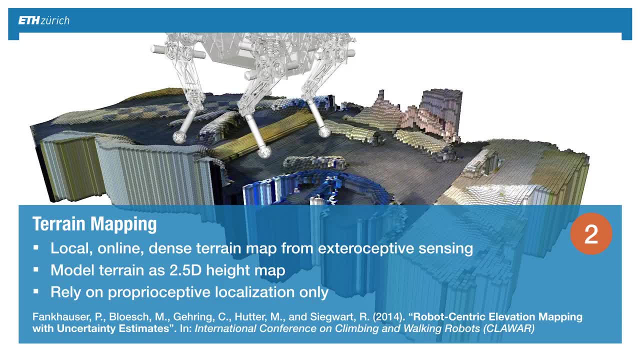 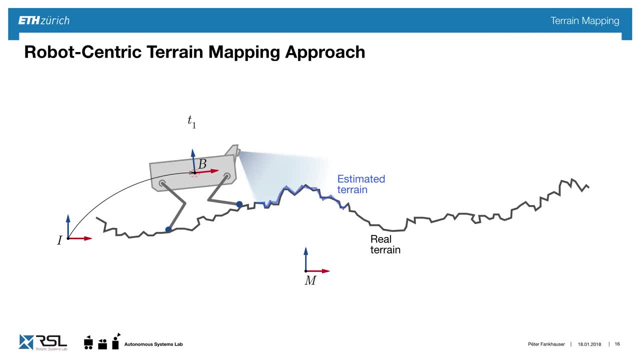 on proprioceptive localization, which makes it much more robust because we don't need an absolute or external localization system. So let's imagine the robot on the terrain at times T1, and as it walks forward, it's now there and we'd like to create the map. 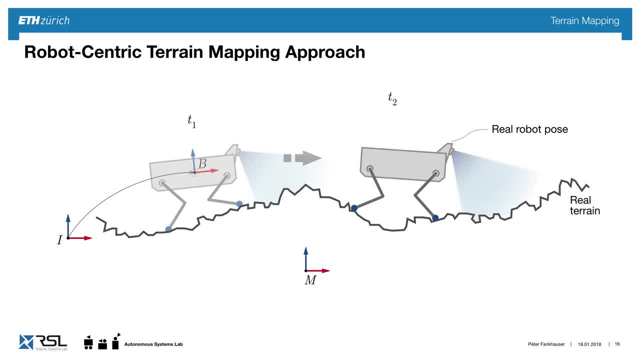 Now, in a classical view, sitting in the inertial frame from the outside. we know from experience and from literature that this proprioceptive sensing, which relies only on inertial and kinematic data, drifts over time in position and yawing angle. 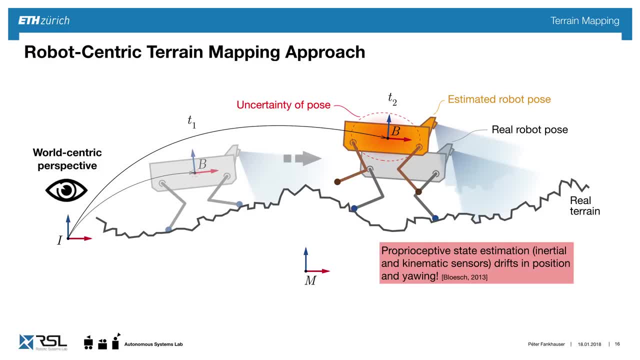 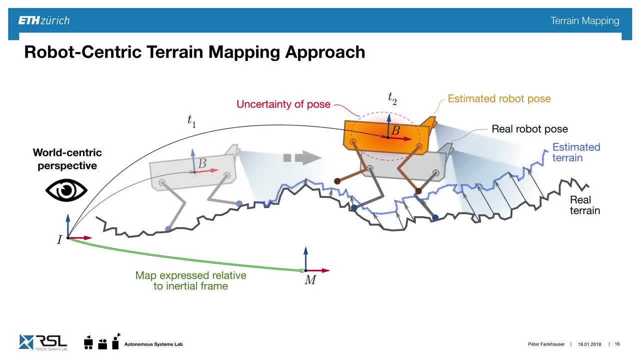 So here the position of the robot as it walked becomes more uncertain, here depicted as the orange robot. And if you do mapping straightforward, we create inconsistency in the map due to that, which are a problem for planning In my work. I propose to take a different approach. 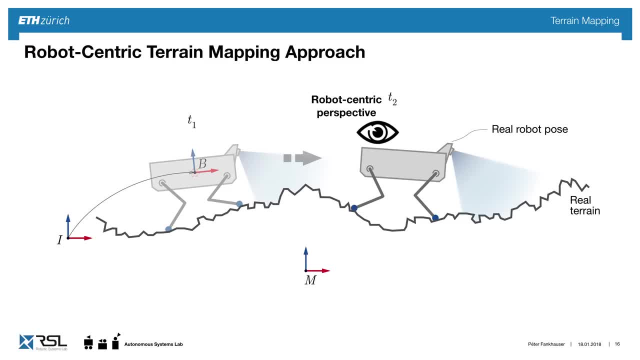 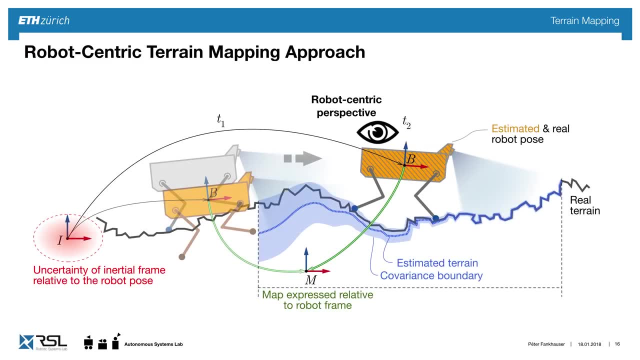 and model the entire thing from a robot-centric perspective. Now we sit in the situation of the current time of the robot and it knows about its position exactly. but the past position of the robot becomes more uncertain. And now, if you do mapping, 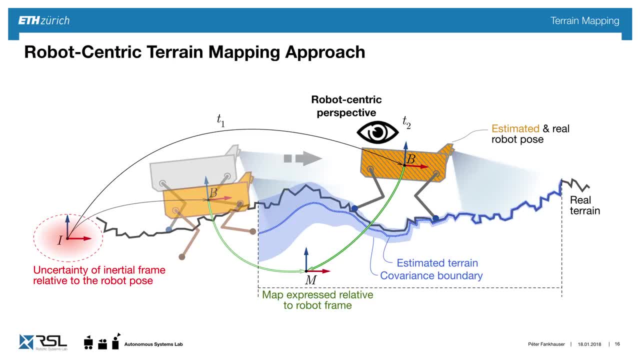 we see that in the front the map is very clear, but the data that the robot has not seen for a while becomes more unclear. And we have- we can introduce these covariance boundaries to upper and lower estimates of where we expect the real terrain to be. 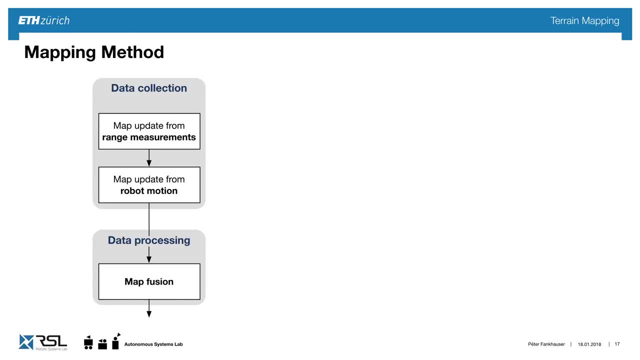 Now formalizing this in my work. I have separated the work in two parts, which is the data collection and the data processing, And I'm gonna go through these steps. First, we have the range measurements and for each cell where we have the measurements, 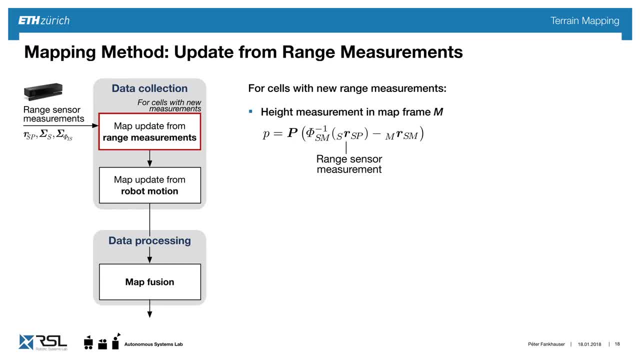 we have to transform it, transform that to a height, which we can do straight forward from the range measurement vector, and transform it to the map frame And then use a simple projection mapping to get the vertical height of it. And for the error, 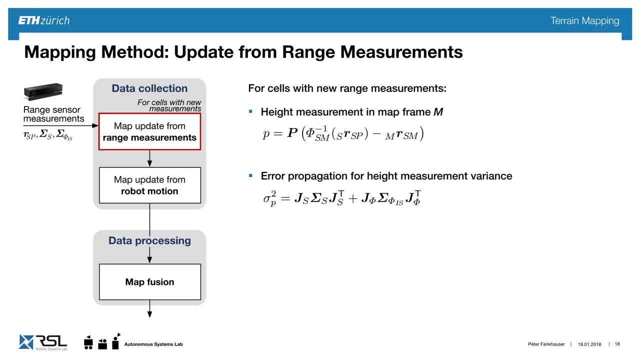 importantly, what we want is to get the error of the cell resulting from the sensor measurement covariance which we evaluated in the part one, and from the sensor orientation covariance on roll and pitch which we get from the legged state estimation. Now, if there's an empty cell, 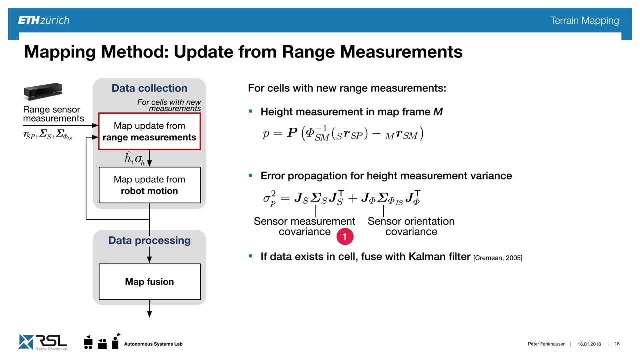 we can fill in this data, but if there's already data, we're gonna fuse new data with existing in the sense of a common filter where we evaluate the new height as follows: And then we have also the new variance for the cell in this common filter. 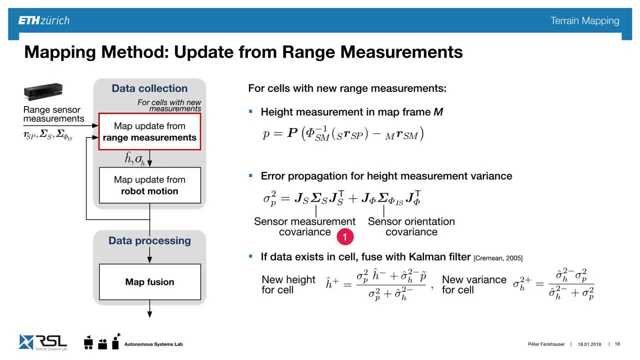 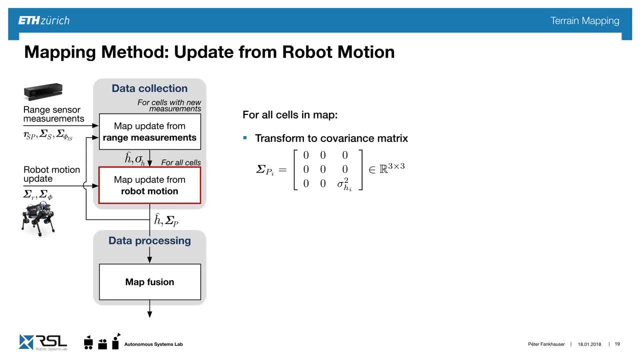 and we can create a consistent map. And this is getting the laser data into the map. And in the second part I wanna introduce the errors that we get from the robot motion And we have to transform the height variance to a full three by three covariance matrix to do that. 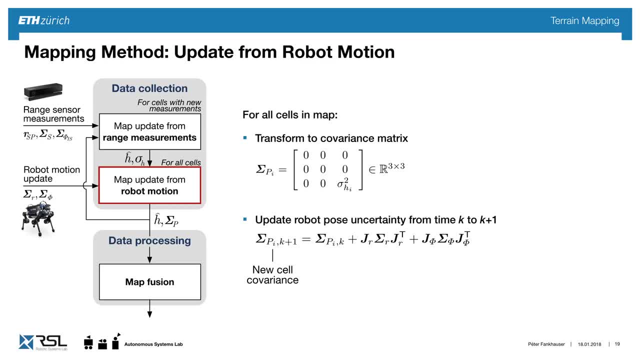 Then we can take the robot pose uncertainty from time K to K plus one and get the new cell covariance out by taking the old, the previous cell covariance and taking this robot pose covariance updates from time K to K one and JSON the Jacobians. 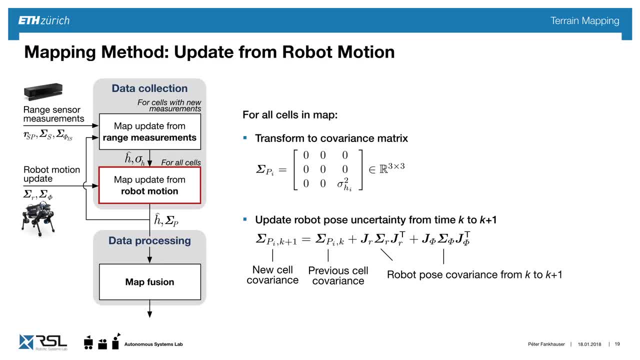 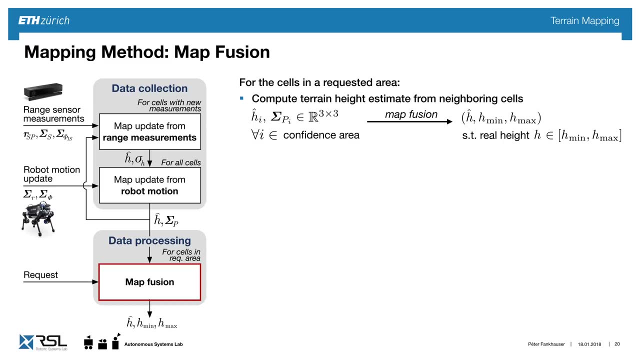 to do the proper error propagation mapping. Now that we have this three by three covariance matrix for each cell and the height, what we really want is to get the height and the lower and upper boundary. So we have to look at each cell individually. 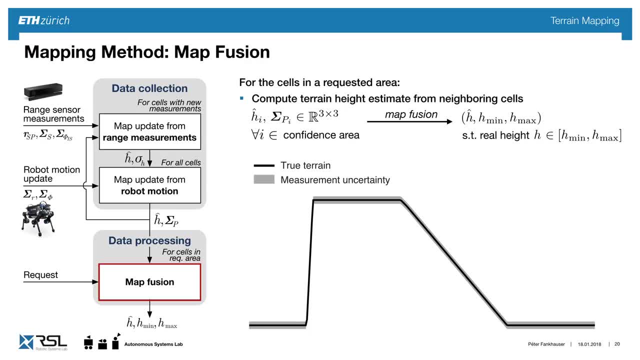 and I'm gonna explain it with the following illustration. So imagine this is a profile cut from an obstacle, from the terrain, and then sample. now one point and we look at the error ellipsoids and create a probability density function which is: 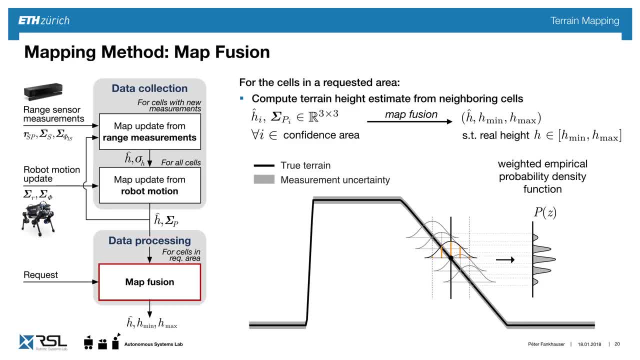 we can integrate it empirically, based on the distance from this cell to the neighboring cells. Now, from this probability density function I can integrate that up and create the cumulative density function, from which then I can sample the first zero quantiles and from this predict the maximum and the minimum height. 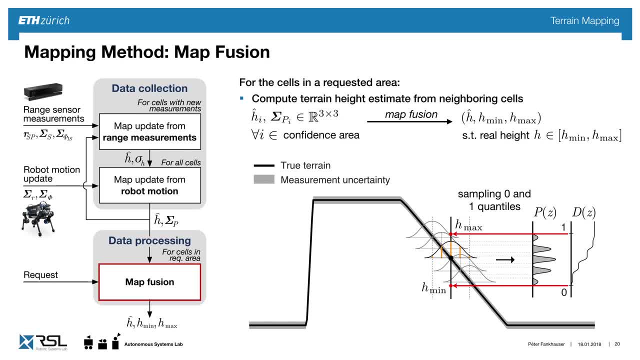 expected to be at this position. Now, I did this for one cell and if I do this for the entire map, I can create this confidence bound. Now the same view here in 3D. this is the original train in the left. 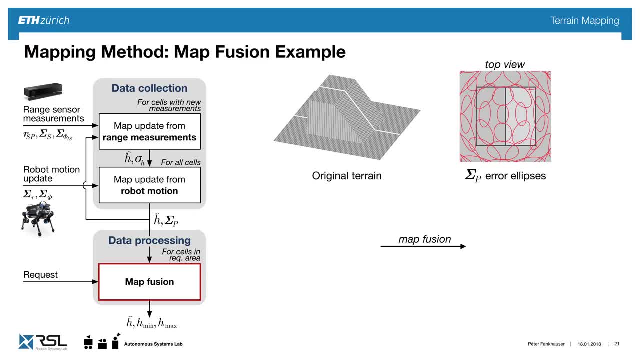 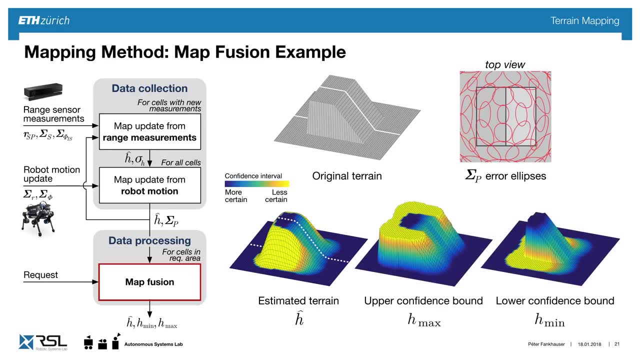 and on the right. I've plotted these error ellipses from the top view And if we go through all of these points, what we get is kind of like this: smooth out terrain on the left for the estimated terrain, and here blue means that we're more certain. 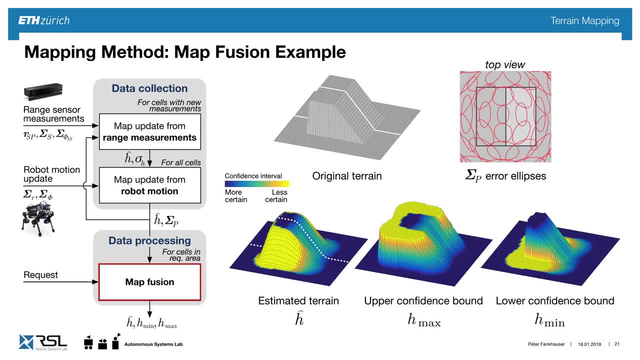 about this sampling point and yellow means we're less certain about it. And on the middle and the right you see the upper and lower confidence bounds which tell us here is the maximum and the minimum expected terrain to be. And, importantly, later we're gonna choose. 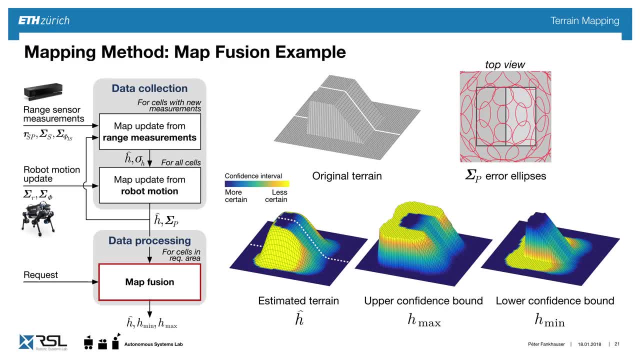 of course, the blue areas to certain areas to step on, because there the robot knows, even though the train is uncertain, there's still certain positions where it can safely step on. Now here's the train mapping in two examples where it does real-time train mapping. 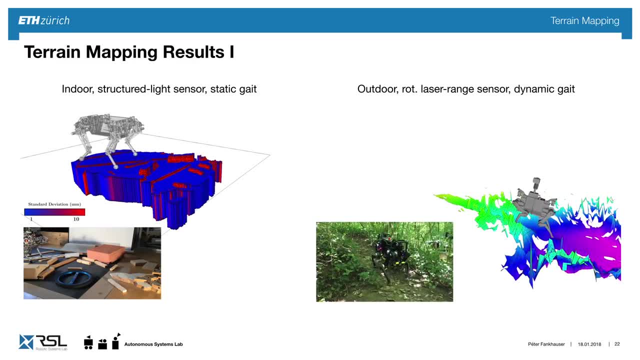 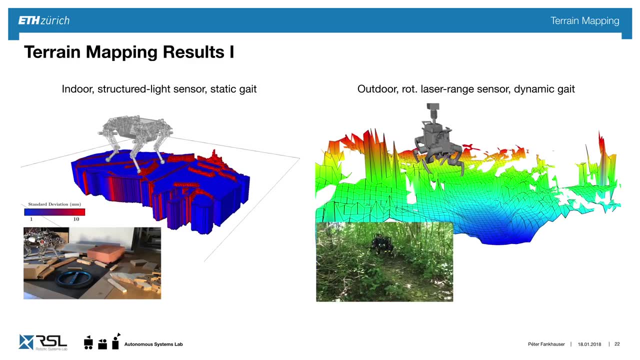 from the left-hand side to use the robot Starlet indoor with a structured light sensor with a static gate. On the right-hand side it's outdoor, complete different setup in a forest with a rotating laser ring sensor with a dynamic tracking gained on a robot animal. 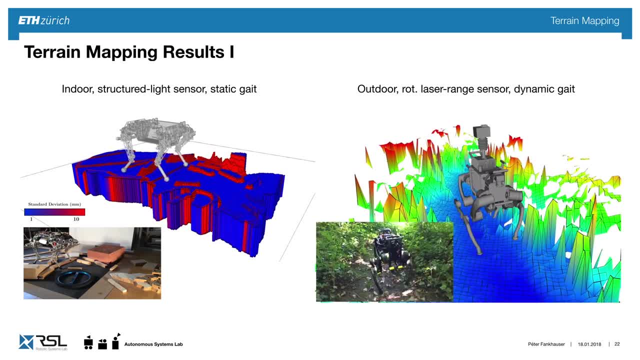 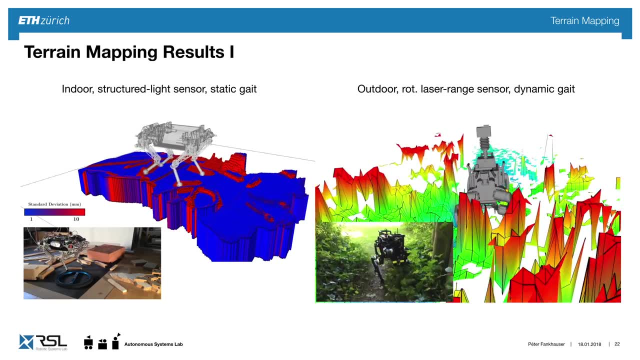 And in both cases same principle, but we see the difference in quality of the maps. Now, to analyze this more clearly, we have done the following experiment: We have created a scene and then scanned it as a ground truth with this multi-station. 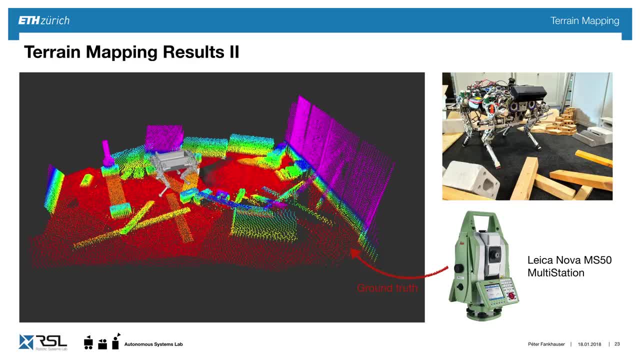 where we create the absolute point clap from the environment, And you see in the video how the robots walk through this and in the front you see the current scan that it currently takes in comparison to the ground truth. Now, when evaluating this, 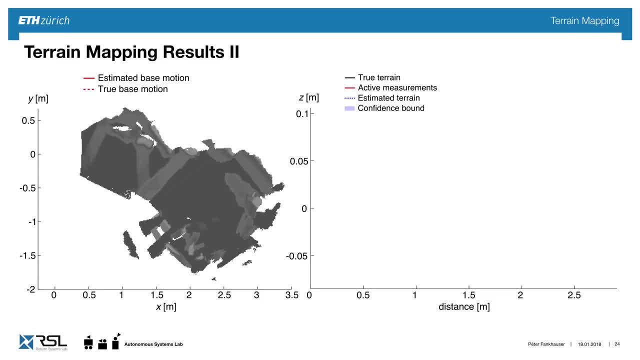 this is a top view now of the train on the left-hand side. What we're going to do, we're going to show how this map evolves and we're going to look at one profile cut and look at it from the side, from the right-hand side plot. 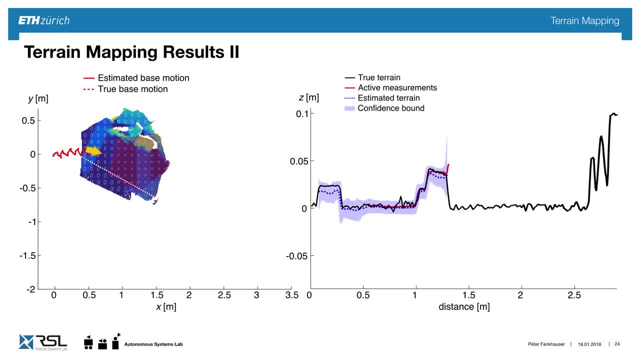 So in the beginning we see that the map, the estimated train, here plotted in blue dots, and the real train in the black line. they are very well aligned. But as the robot walks we notice in the back that the train, the estimate, starts to drift away. 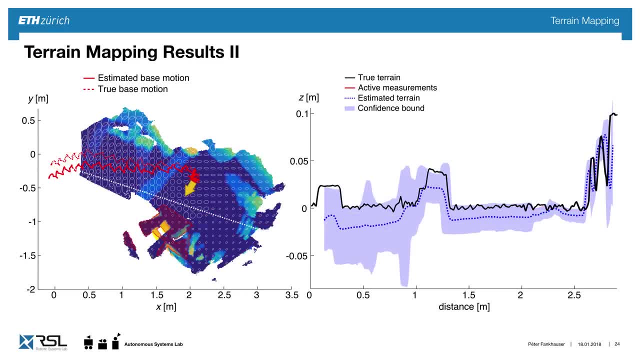 And in the final picture we see that there's quite an error between the estimated and the real terrain. However, the method is shown to work because the true train lies well within the confidence bounds of the estimated train. So now that we have the mapping, 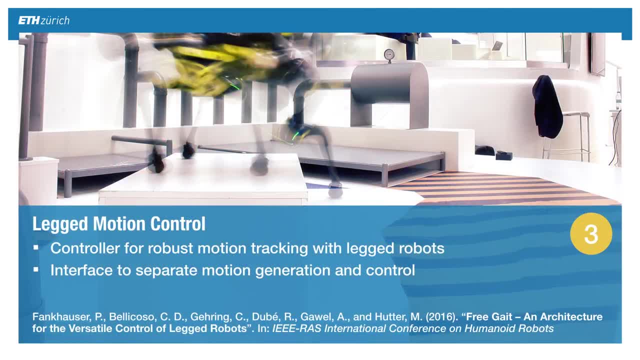 I'm going to show you how we control the robot. And here I'm going to show you how we control the robot. And here I'm going to show you how we control the robot. So our goal was to create a controller for the robust motion tracking of legged robots. 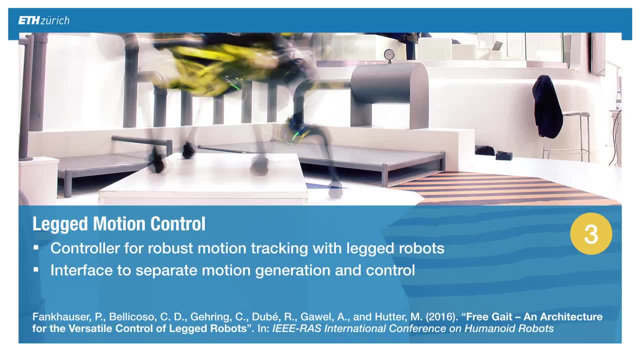 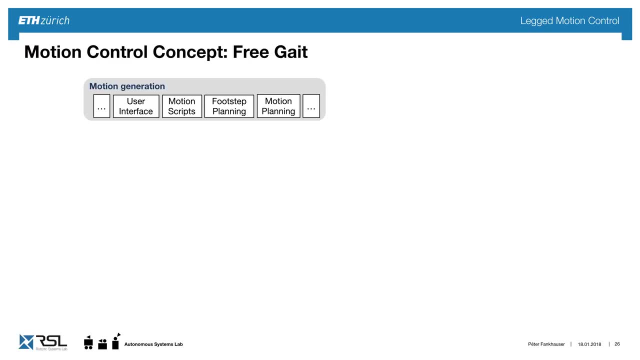 and really to focus in on creating an interface which separates the motion generation from the control. So how do we control the robot? Typically we use an interface such as a joystick computer screen or we use motion scripts that we can replay in the robot. 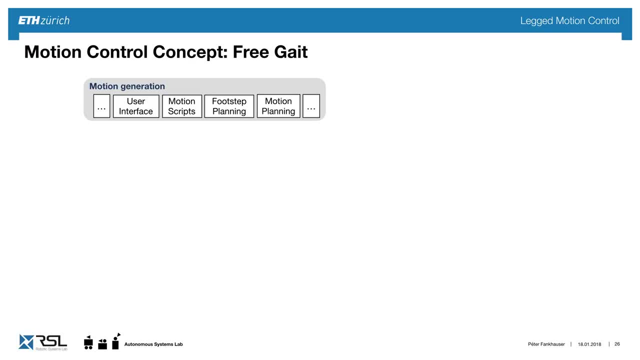 Or if we go one step further, we can create footstep planners or full motion planners to do complex motions, And then we somehow interface this with the controller which does the real-time tracking of the robot. And here we see, classic, the state estimation controller. 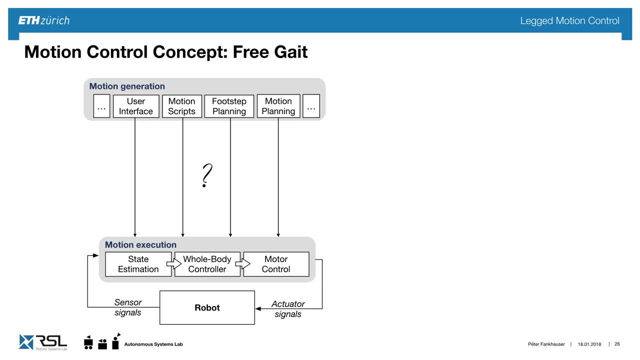 and then, in this real-time, it tracks the desired motion. But every time we create the new interface it's error-prone and it's a lot of work. So I propose a universal interface for legged robot to control, which I call the FreeGate API. 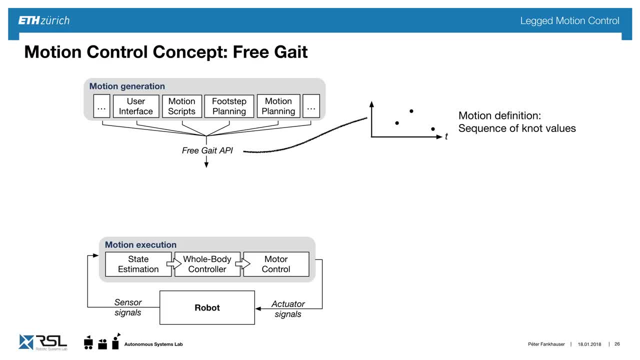 Here. this is a unifying interface where I define the motions by a sequence of not values And in the second step I can transition from the current state to the desired motion and spline through these not points for trajectory generation, Then for the real-time control. 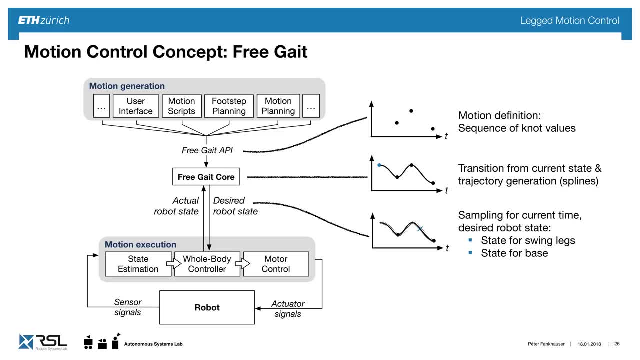 we sample this trajectory at the resolution that we need And finally we get to the control of the state for the swing links and the state for the base. I wanna focus a little bit on this FreeGate API, which is a very important part of this work. 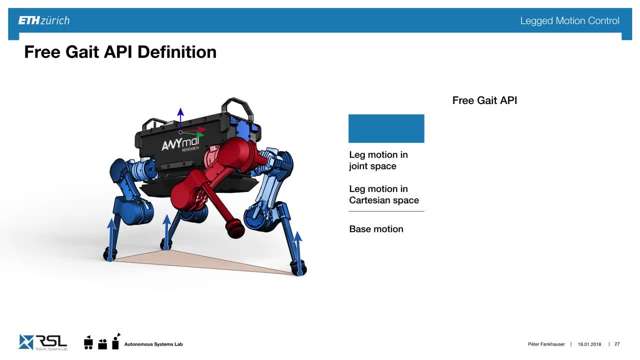 The FreeGate API consists of two main motions. One are for the leg motion, which can be defined either in joint space or partition space for the end effector, here shown for the right leg, And base motions, where we define the position orientation. 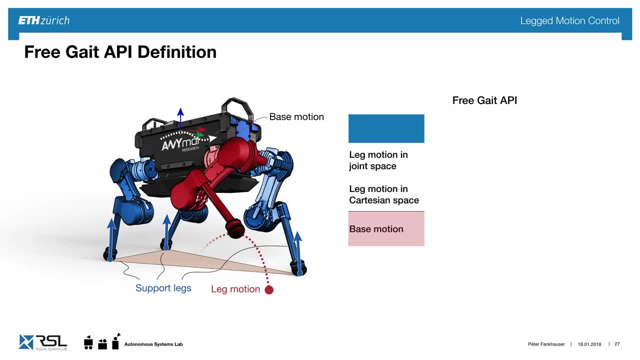 and velocities of the torso of the robot, which then automatically mean that the legs that are in ground are determined through this motion. Now there's different types. I can send this command and one is a target where I simply send: go to this position, your leg on the base. 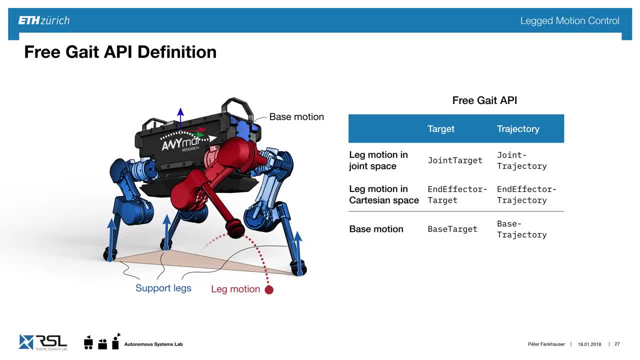 And then from a complex motion I can do full trajectories. And I've created this library with a set of automatic tools which means I can send it a target foot location in the case of a footstep, and the robot would automatically figure out. 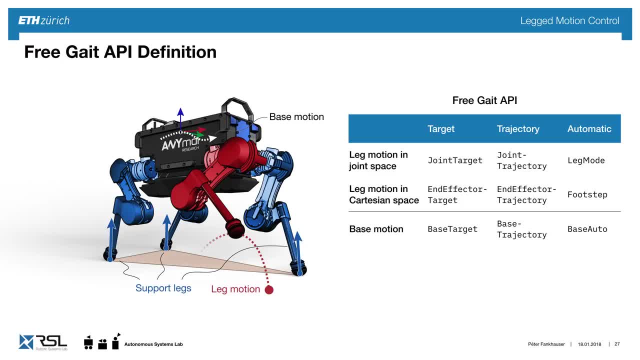 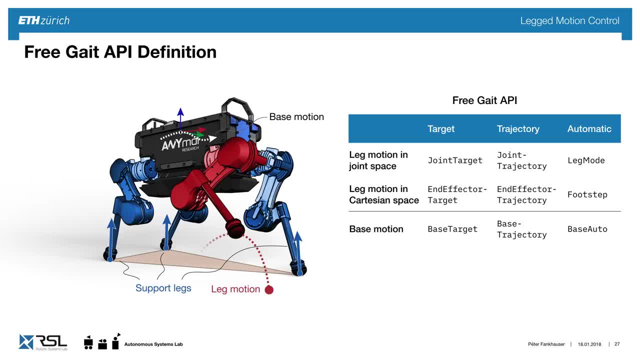 Now, from these elements of API parts, we can mix and match our commands together. And here's a simple example of the robot's walking. It uses the base auto command to make sure the base is aligned correctly and uses a simple footsteps to walk. 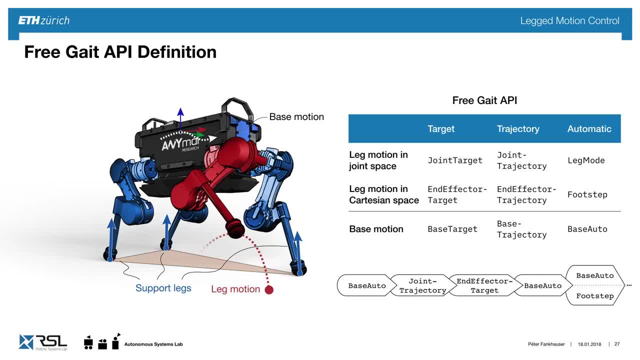 For another example where we use a Journey Trajectory and here would turn around the leg And, for example, change the configuration, use the end effector to touch something. So we can really, with this tool, take these elements and parallelize them as we need them. Importantly, all these commands can be represented in the 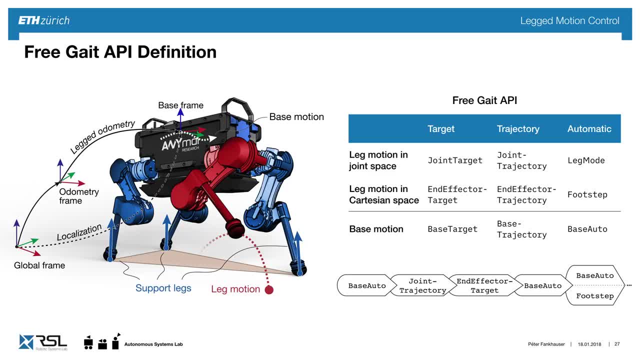 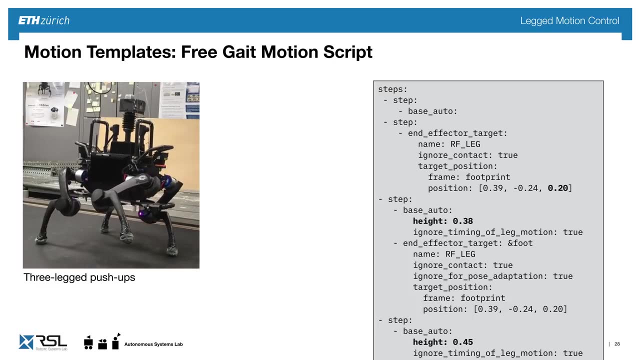 arbitrary frame, which is important for the task at hand. With this tool, we've created an API for the versatile, robust and task-oriented control of legged robots, And I'll illustrate this with the following example. Here, we asked the robot to do three legged push-ups, where one leg should 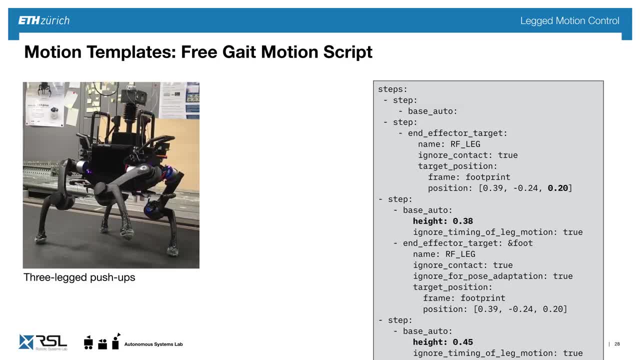 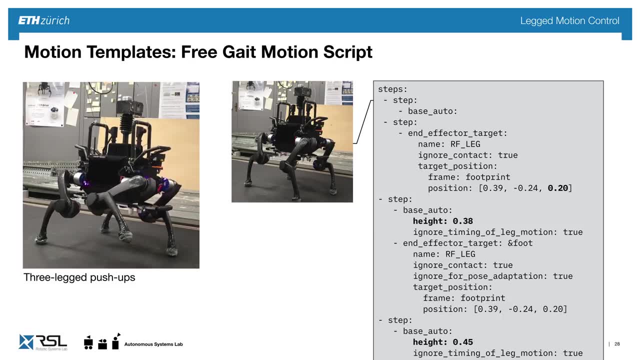 stay in the air And on the right-hand side you see the motion script that we used to program this. So first we used the base auto command to move the base to stable position. Then we tell it the right front leg should move to 20 centimeter height in the footprint frame which is defined. 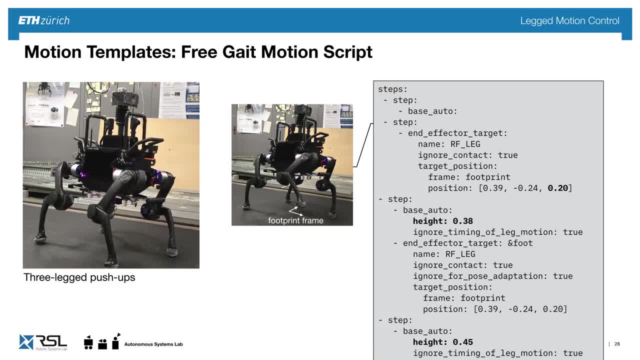 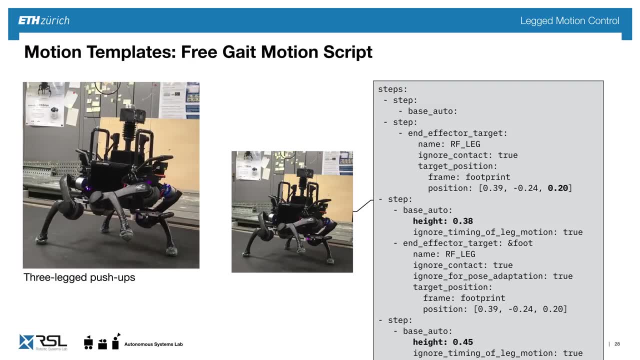 between the legs. Then we simply ask with the base auto command to move your base to a height of 38 centimeters by keeping the leg at the same position, And then this motion of adapting the leg to stable position. And then we ask the robot to do three legged push-ups, where one leg 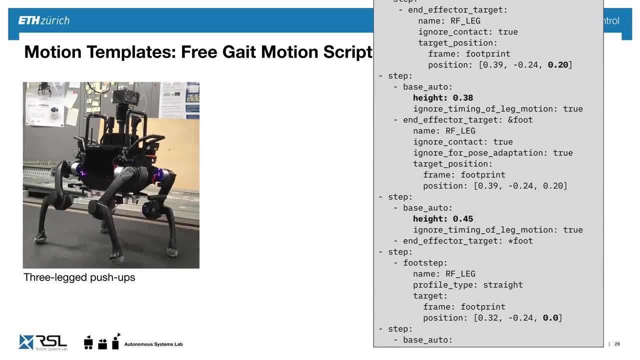 should stay in the air, And on the right-hand side you see the motion script that we used to program this, And here we asked the robot to do three legged push-ups, where one leg should stay in the position, of course. automatically We move the base up and down here to 45 centimeters and then 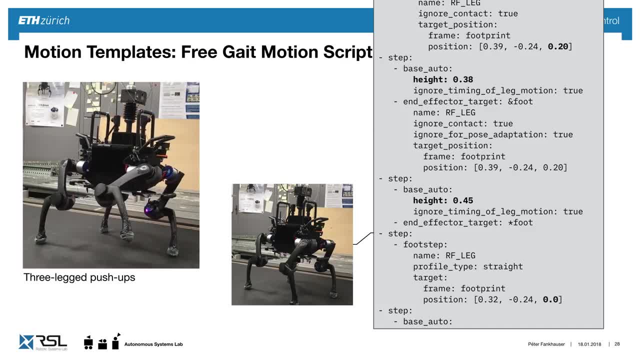 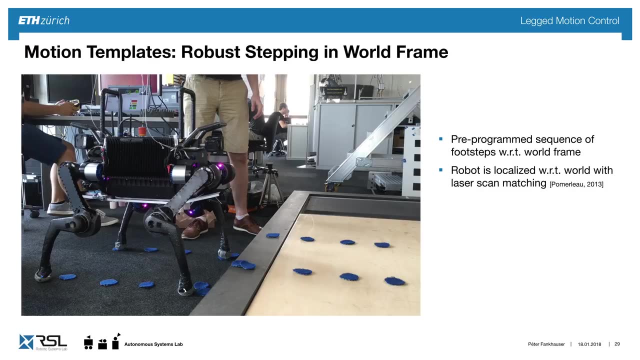 lift it again down in straight profile type to the ground. So with these 35 lines of codes, I've already programmed the robot to do this complex motion through this API. Now, when working in real environments, it's important that I can track the robot's motion. 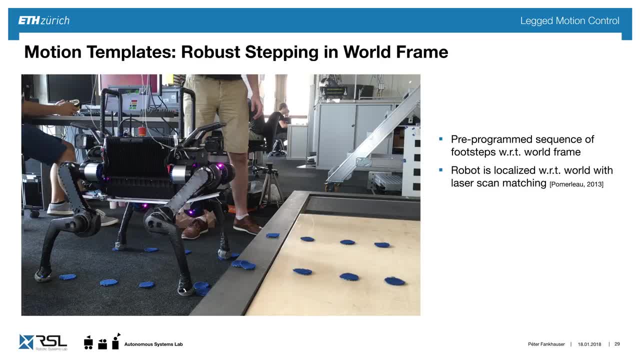 with respect to the environment accurately. To show this, we've pre-programmed the sequence of footsteps here showing us blue dots on the ground in the world frame, and the robot is localized with respect to the world frame with the scan matching with the laser, And we're gonna start multiple runs from different positions and show. 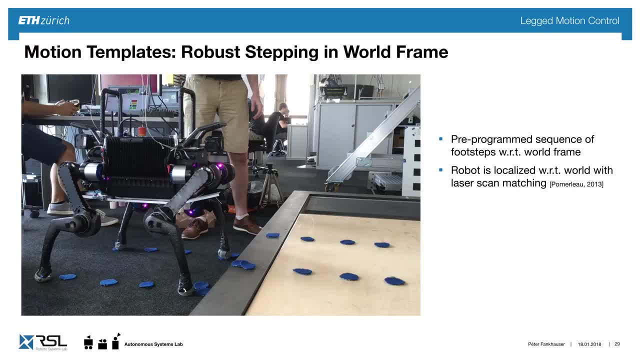 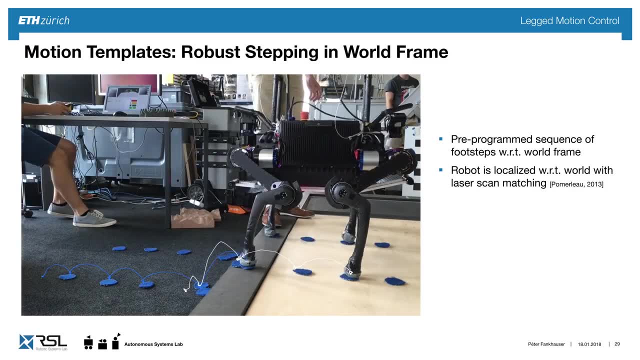 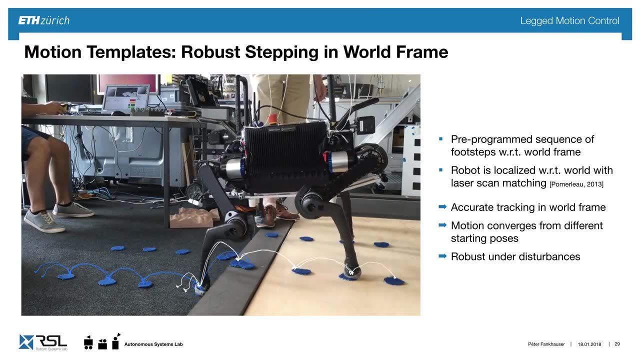 the result. We can see that after one step already, the robot steps onto the desired locations and then, repeating this from different positions, we can see that the motion converges very quickly and even it's hard to see, but the person that pushes the robot- or later we use a pipe on the ground to diverges from the. 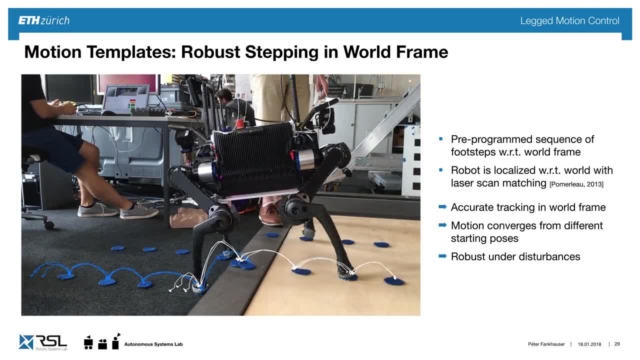 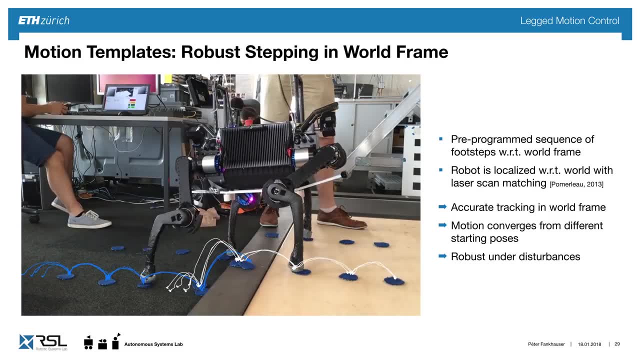 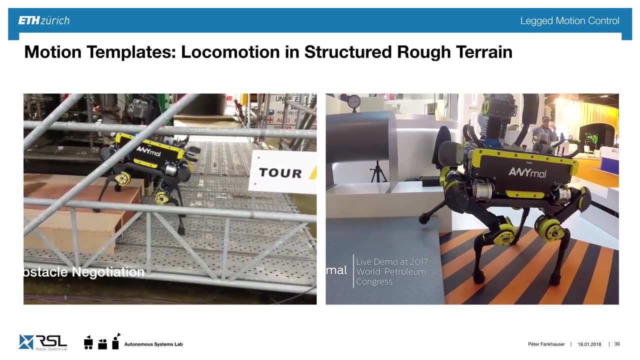 desired footsteps so the motion can be tracked robustly, even on their disturbances. We use this in several projects, such that in terrain that we know of structured rough terrain, and here we see the robot choosing from a set of templates to climb over obstacles, climb over gaps. 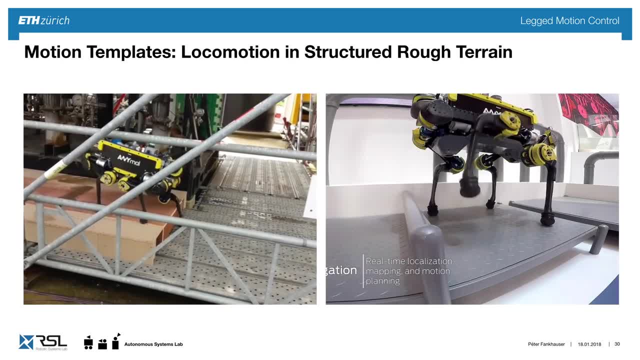 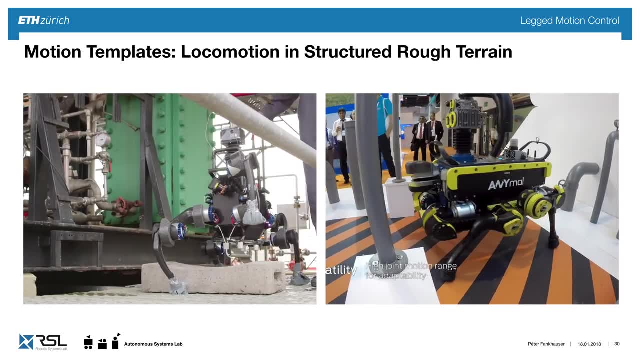 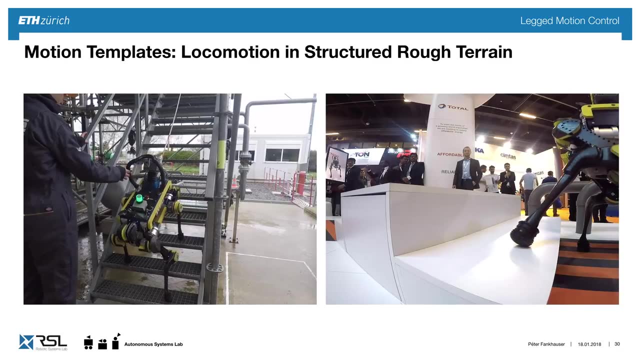 and either its known from the environment or the user chooses an adequate motion. here we rotate the legs to go over big obstacles and finally we can also climb very steep industrial stairs which are steeper than 45 degrees. Now, since this is so flexible, you can go ahead and, for example, change the height. 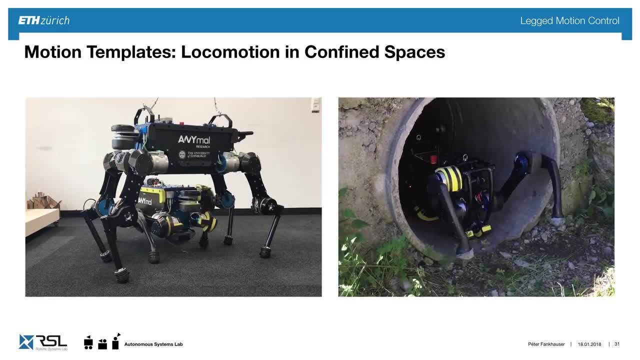 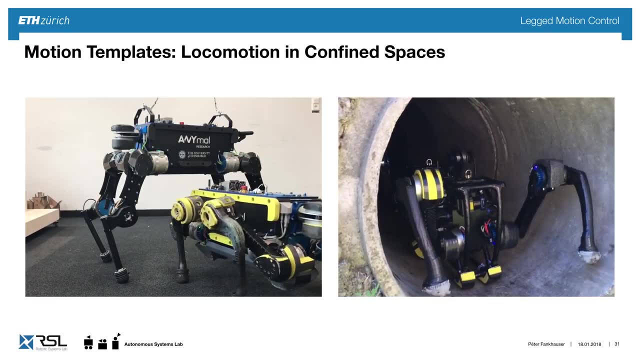 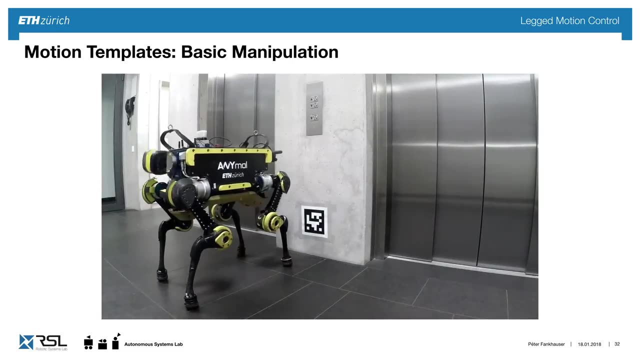 to make the robot crawl or by changing it's legged configurations. with this spiderlike, we can really go into pipes and use this motion flexibility of the robot robots to achieve these maneuvers. Going one step further, we can do a simple manipulation And here we see the robot pressing. 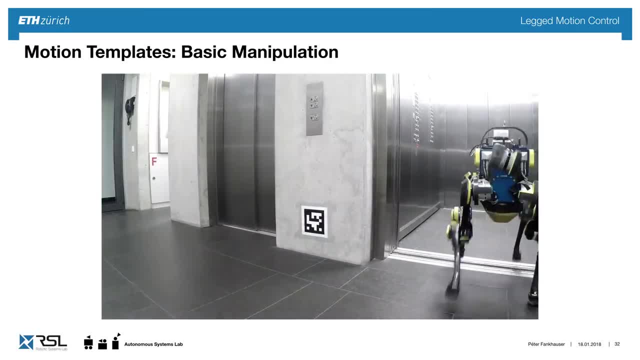 the button of the elevator And in this task, we use the April tag, which you see in the video, in order to determine the position And simply told that to the FreeGate API. this is where we want the robot to push. 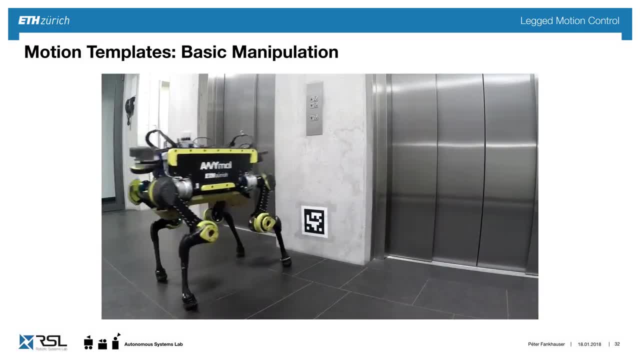 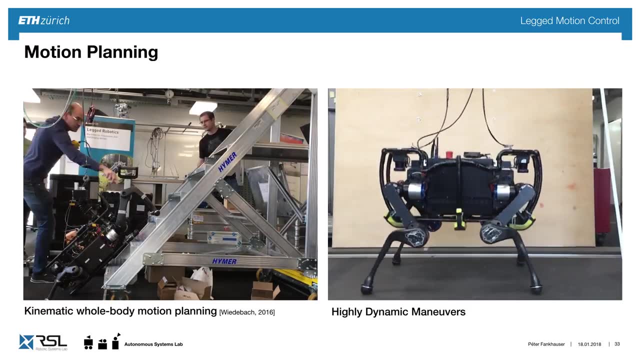 And these are template motions from which we can choose in the library. Of course, this interface is also meant as an interface for motion planning, And on the left-hand side is work I've done with my student where we did kinematic whole-body motion planning in order. 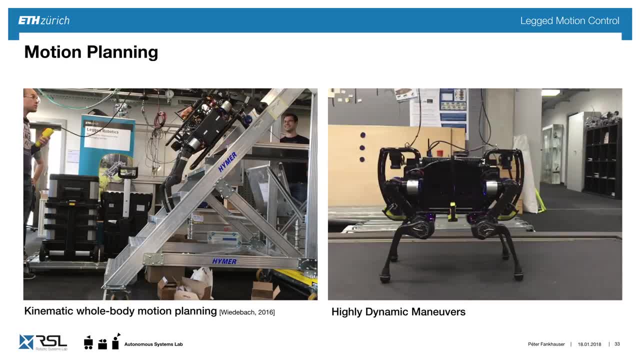 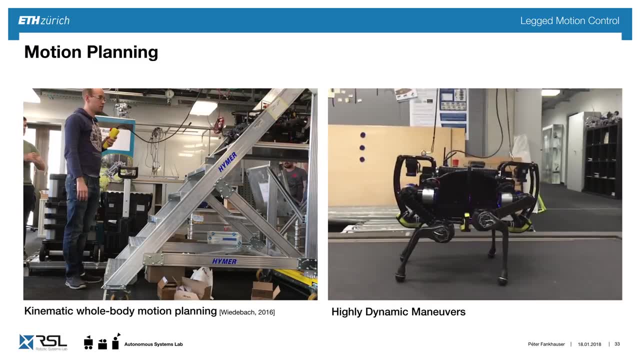 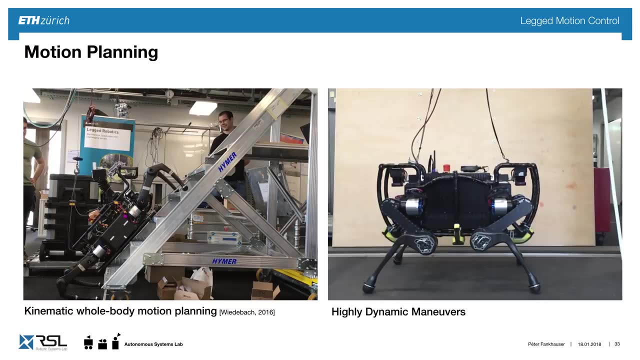 to climb these stairs. We can also do highly dynamic maneuvers on the right-hand side, where we see the robot jumping and rearing. Now that we know how to control the robot, our goal is to put things together and create a locomotion planner that uses the map and these control. 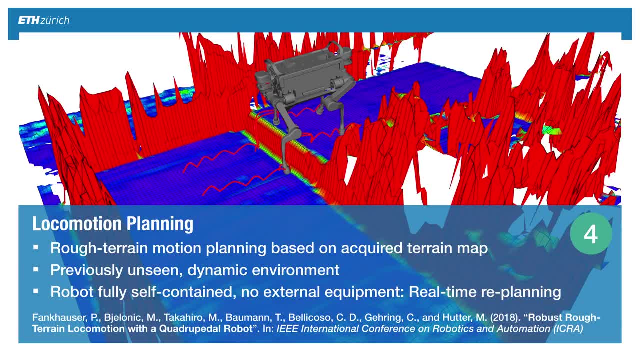 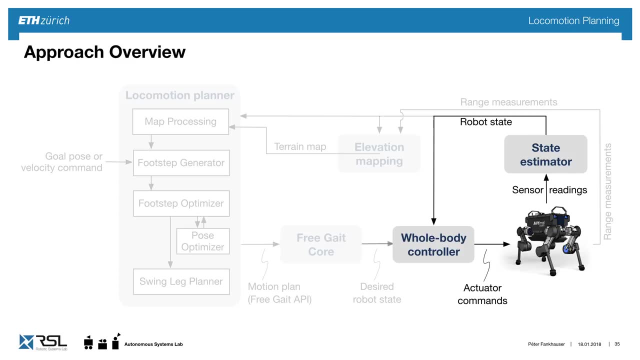 abilities to run over the train. The goal is that the system works in previously unseen dynamic environments, and everything should be fully contained. So there's no external equipment and all the re-planning happens in real time. This is the overview of the entire scheme. 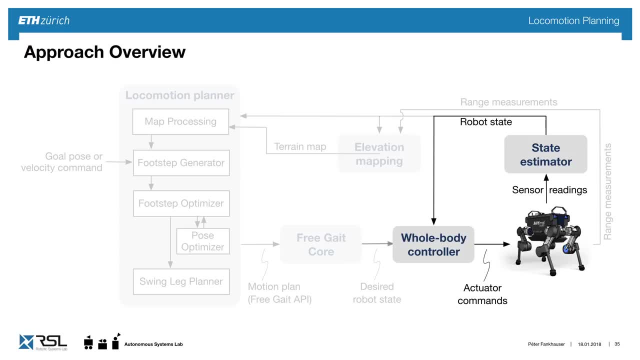 I'm going to go through it step by step. So here again we see the classical control loop of state estimation whole-body controller And we've seen in part one and two how we use the distance, the distance sensors, in order to create the consistent elevation. 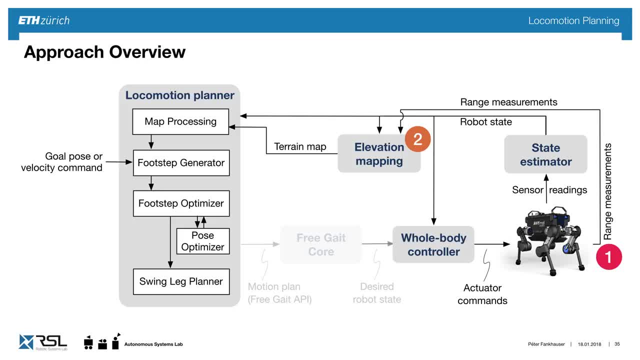 map of the terrain. Then the locomotion planner takes the terrain data and the current position of the robot to run through a set of processes in order to create a free-gate motion plan, which is then translated, as we have seen in part three. 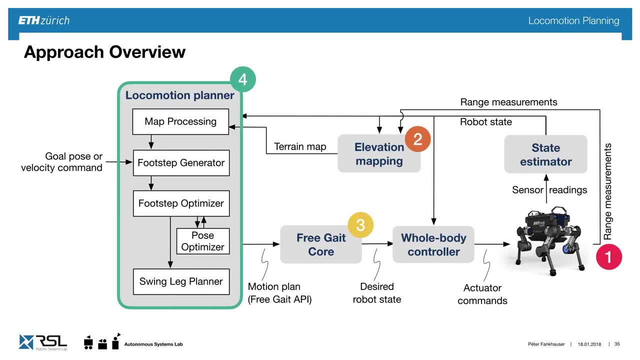 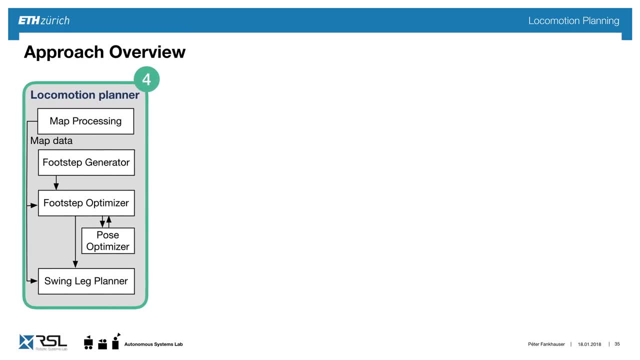 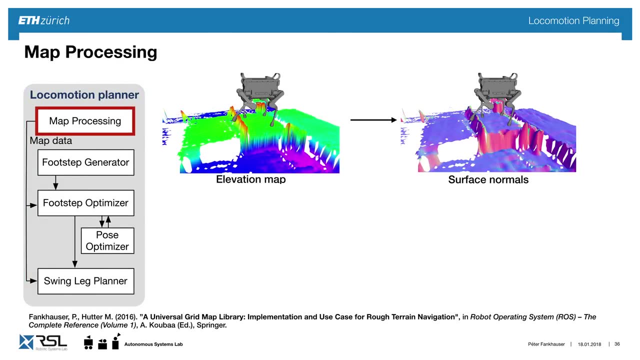 to the whole-body controller And I'm going to focus now on the locomotion planner in this part. I'm going to go through it step by step And I'll play with this So when we get the elevation map we can process this. 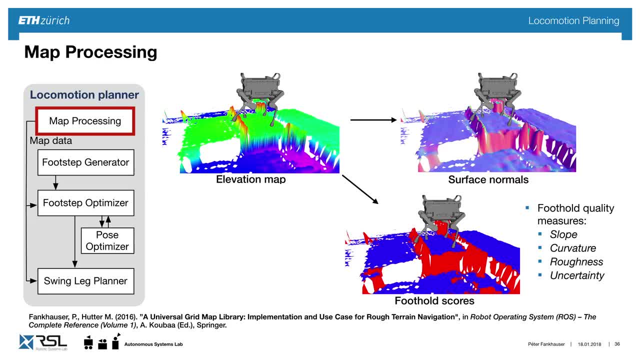 and check for every patch and figure out, for example, the surface, knowing which will be important later. We can process it with different quality measures, such as slope, curvature, roughness, of course, the uncertainty in the terrain to create a foothold quality measure, telling us where is it. 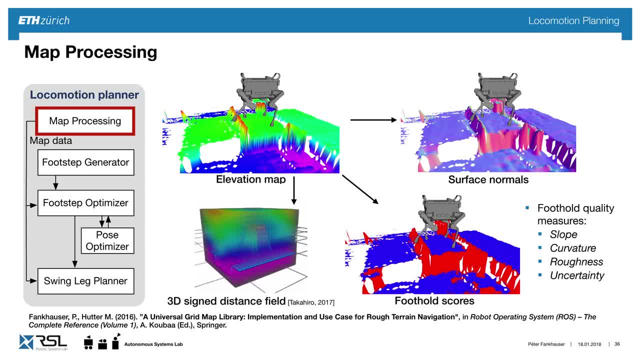 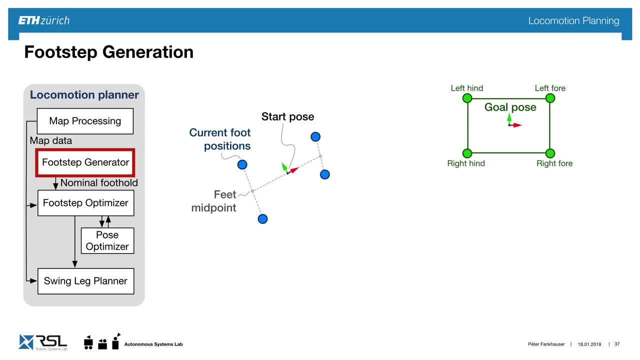 a three-dimensional signed distance field in order to do fast collision checking. Now, first we wanna generate sequence of steps, and here's a top view. On the left, we see the robot standing in an arbitrary configuration and on the right we see the goal pose. 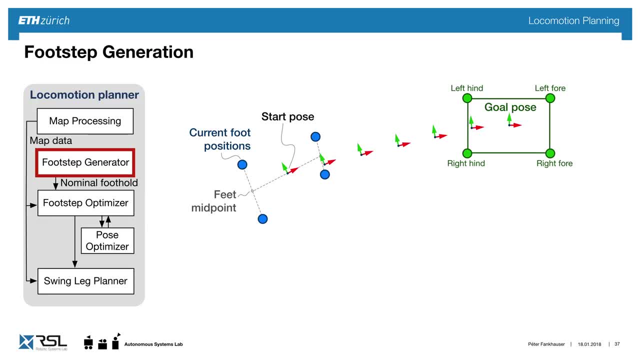 And the process works as follows: First we interpolate a set of stances between the start and the goal, and then just move one stance ahead and choose the appropriate leg, which gives us the first step. In the next step, we do the same thing over again. 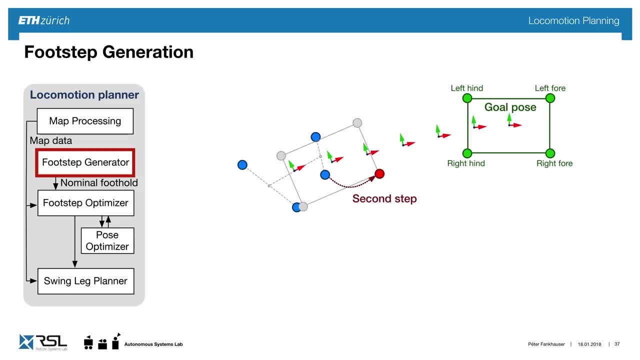 interpolate, choose the next stance and choose the second step. Now, if we do this, we can start, of course, from any configuration, which is nice, But also, since we do recomputation at every time, this motion converges to a skew. 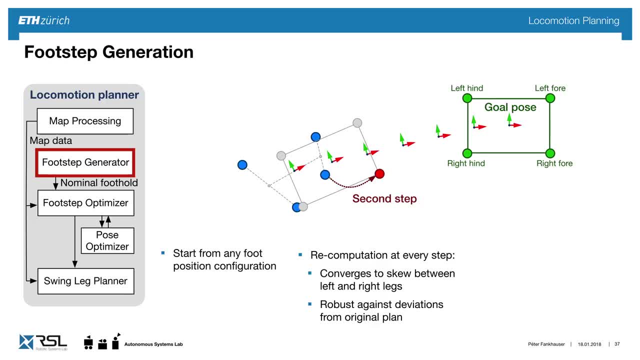 between the left and the right legs, which is important for stability and speed during locomotion, And also because we do recomputation every time. it's robust against deviation from the original plan And finally, it's nice. this motion generation always ends up in a squared position of the robot. 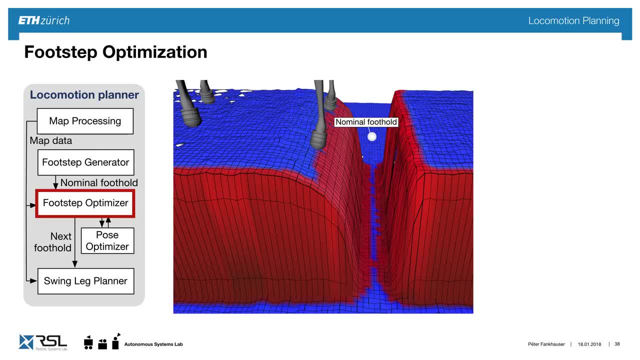 Now imagine the robot stands in front of this gap and the nominal foothold tells it to stand right there in the gap. So now our goal is to adjust these footsteps in order to find a safe locomotion over the terrain. So we sample in a search radius all the candidates. 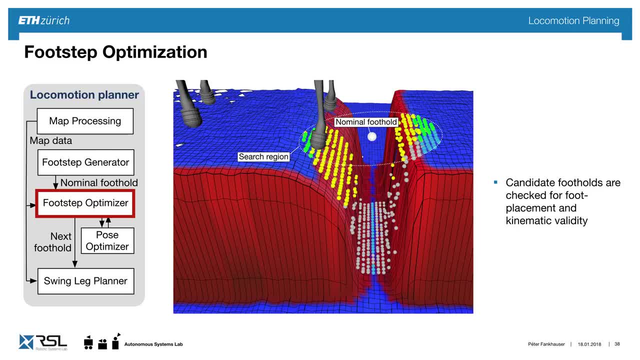 and we can categorize them. First, we have train. we have footsteps candidates, which are invalid from the terrain but would be actually reachable by the robot, like here the yellow ones, Or down there we have valid blue areas. 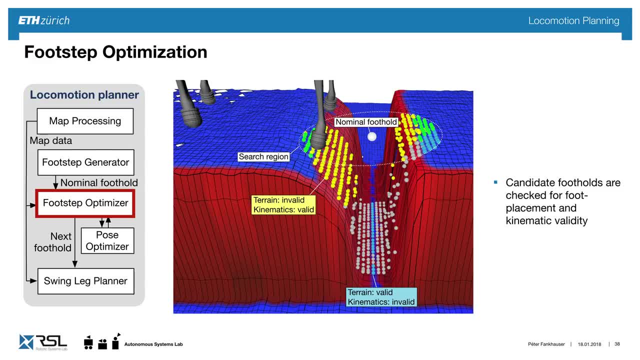 which are fine to step out but are not reachable by the robot. And finally, we have positions which are both valid from a terrain and kinematics point of view, And we choose the closest point to the nominal as an adjusted foothold. 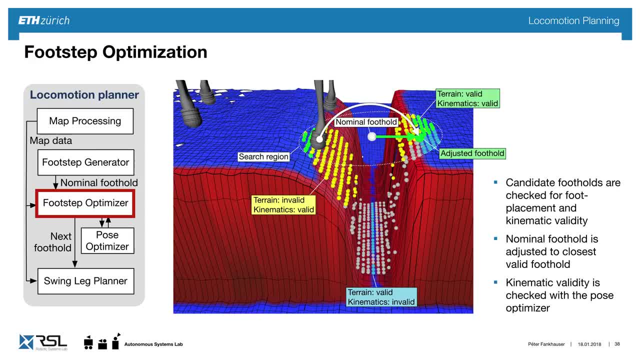 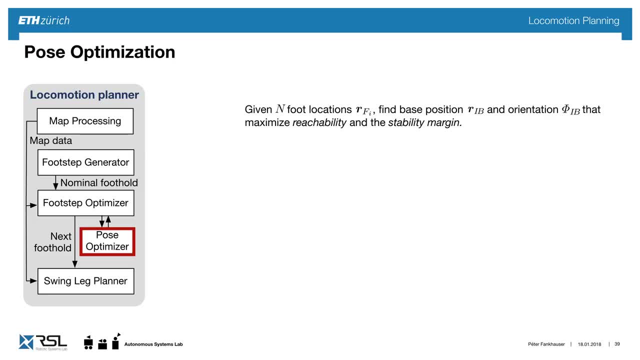 Now we have to check this kinematic reachability. but how do we do this? This is done in the so-called pose optimizer, where its task is given n foot locations to find the robot's base position and orientation That maximizes the reachability and stability. 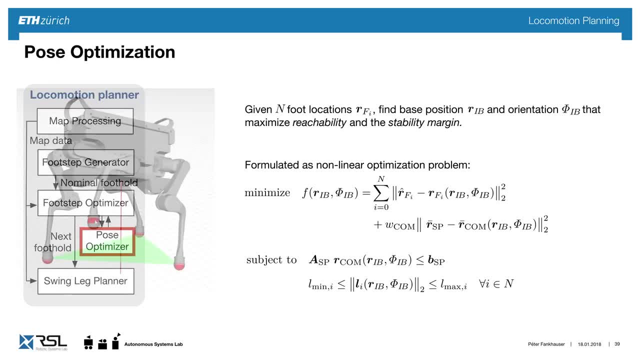 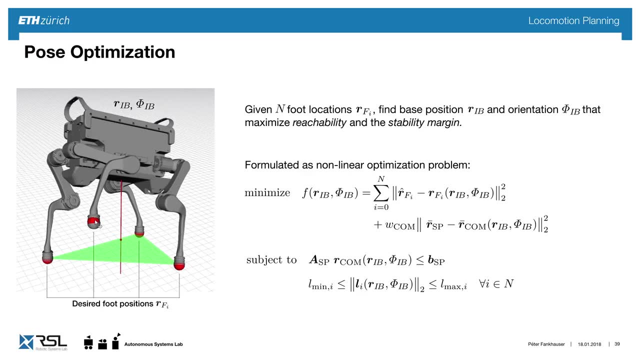 So in the image the goal is really given those red dots at the feet to find the robot pose position and orientation such that the legs can be reached and the robot is still stable And we can formalize it as a non-linear position. 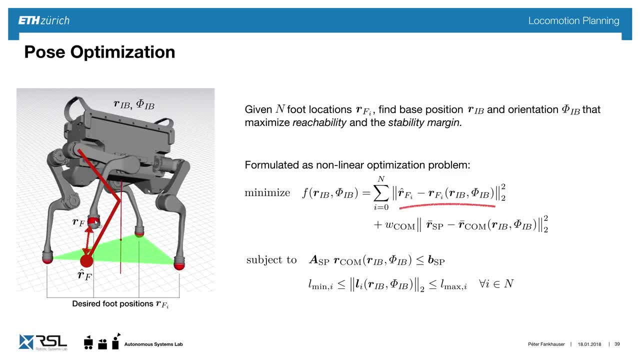 a non-linear optimization problem where in the cost function penalize the deviation of the current setup to a default kinematic configuration, as shown Here- the difference between the foot and the foot in the default configuration- And then we can increase this ability. 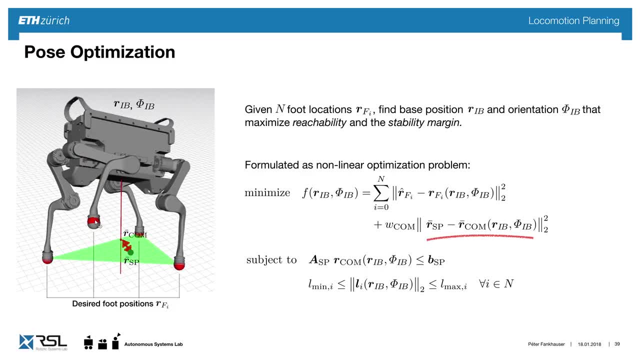 by penalizing the center of mass deviation from the centroid of the support polygon as shown in the support polygon. we've groomed up Now to constrain the solution. we add two constraints: stability constraints to make sure that the center of mass is within the support polygon. 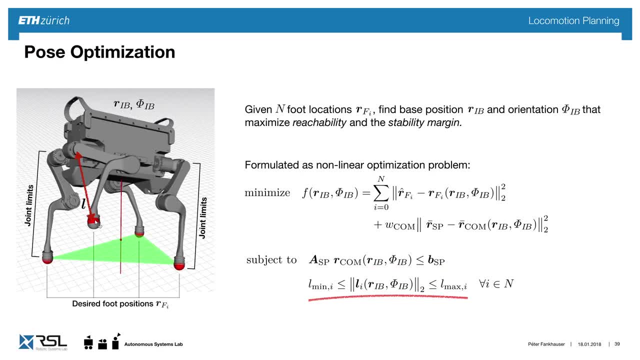 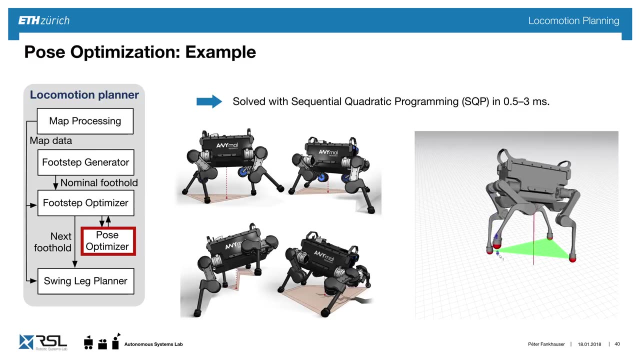 and the joint limit constraints which makes sure that the robot doesn't its legs don't overstretch or go too close. So we can solve this problem very efficiently as a sequential periodic program in roughly open five to three milliseconds on the onboard PC of animal. 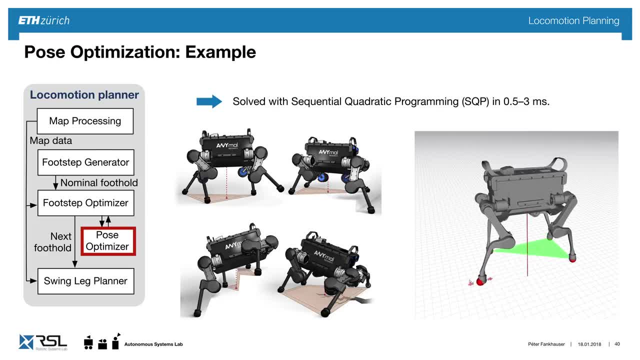 On the left-hand side you see a couple of examples: only, given those footholds, how the optimizer finds these solutions which fulfill the kinematic instability constraints. On the right-hand side, you see an interactive demo where I drag the foot around and the pose of the robot is automatically adapted. 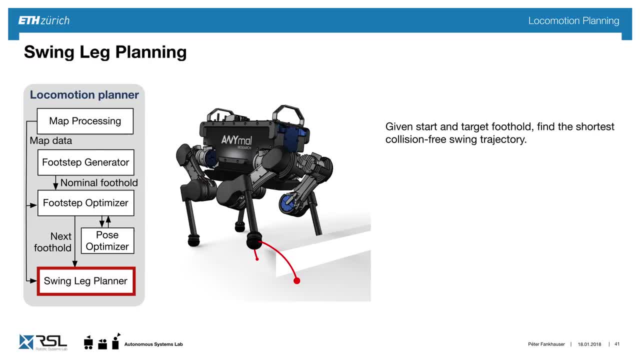 Now that we have the adjusted foothold, or in the last step, the goal is to connect the start and the target location with the shortest collision-free swing trajectory And since we have parameterized our swing trajectory as a spline, we can optimize over these knot points. 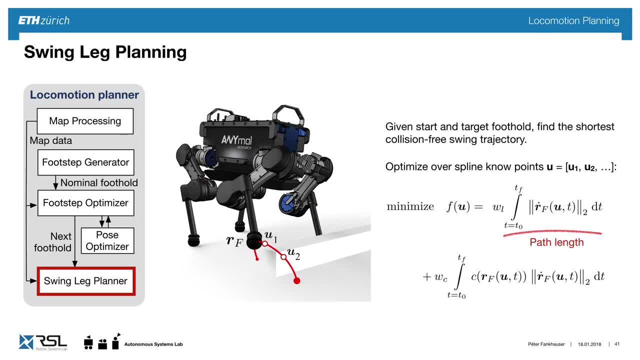 And we do this in a minimization problem, where the goal is to minimize the path lengths while making sure we don't run into collision- with help of a collision function which is based on the signed distance field that we generated from the elevation map, And here we use this term to normalize it. 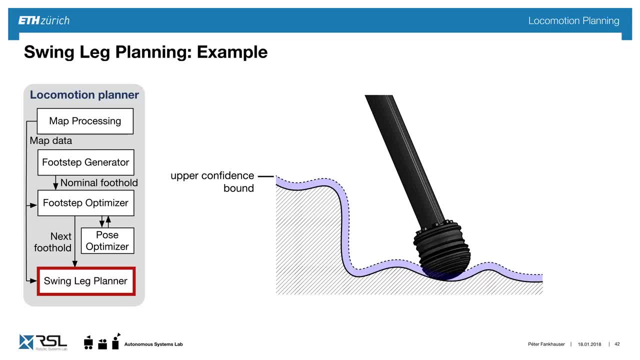 through these collision fields. Now here's an example where we have the terrain from the side and the robot standing on it And we have a terrain with a low confidence bound So typically. and then the signed distance field, which tells us how close we are to the obstacle. 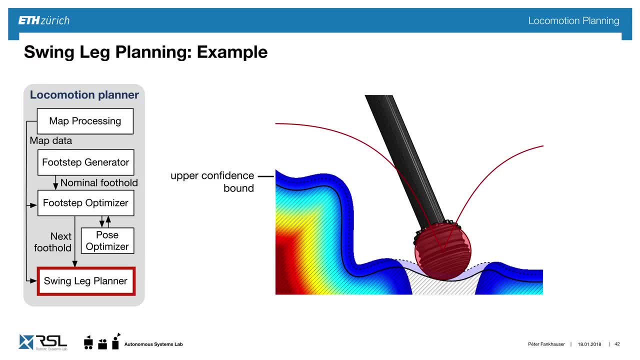 And then a typical solution in this case would be that the robot smoothly goes over the terrain but is collision-free. I imagine we don't know that well of the terrain and the confidence bound is much higher, For example for a hind leg. 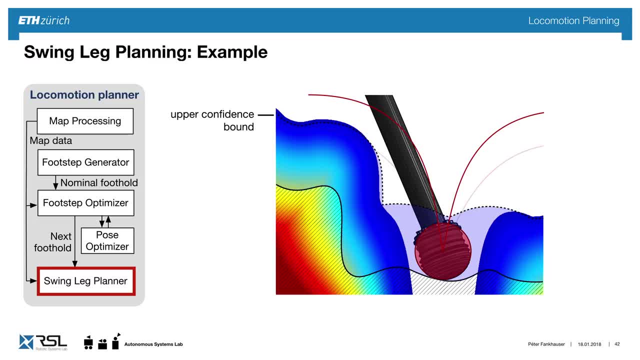 then the collision field is bigger and the solution gives us a much steeper path trajectory of this swing leg, which is nice in an uncertain area where the robot would step much more carefully from top down in order to make sure it doesn't collide with the environment. 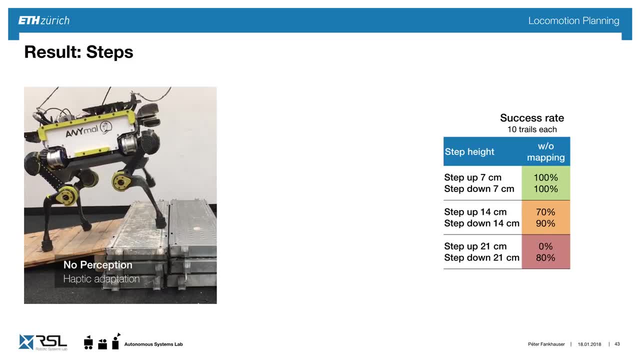 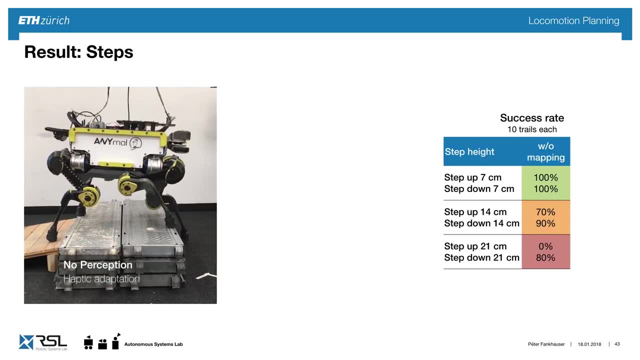 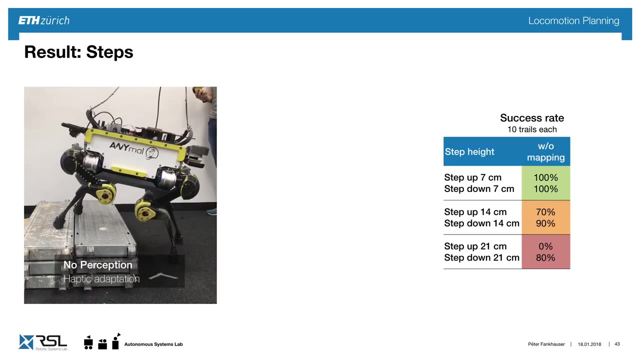 Now, putting things together, we did a comparison with the blind reactive walking that we implemented On the left-hand side. the robot walks blind, takes big steps and has only to feel the ground through the contact forces And, like we see in the success rate. 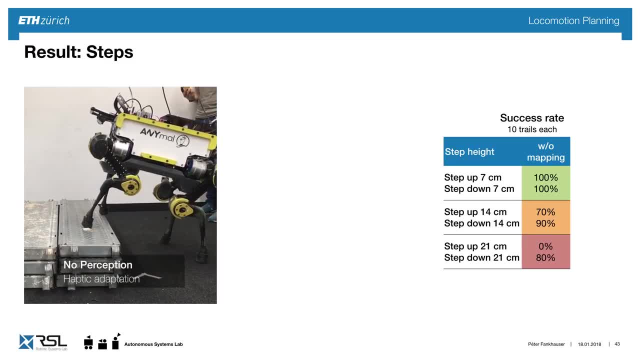 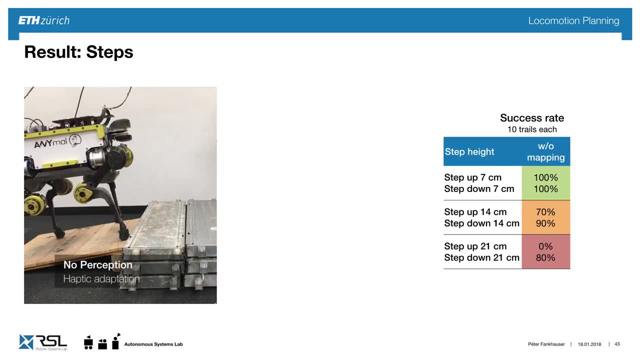 we see that up to obstacles of 10 centimeters this works well, But if we go up to higher obstacles, this is gonna simply fail. that we also needed to run to actually walk up on this obstacle And comparison on the right-hand side. 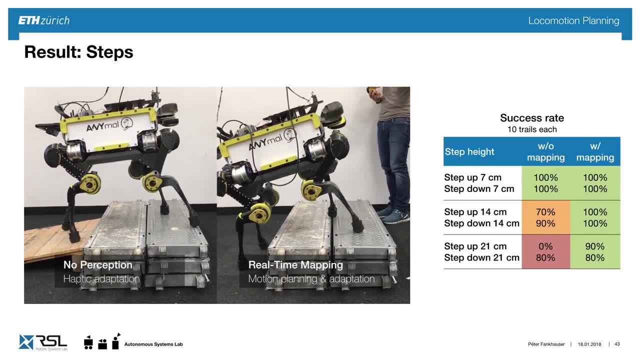 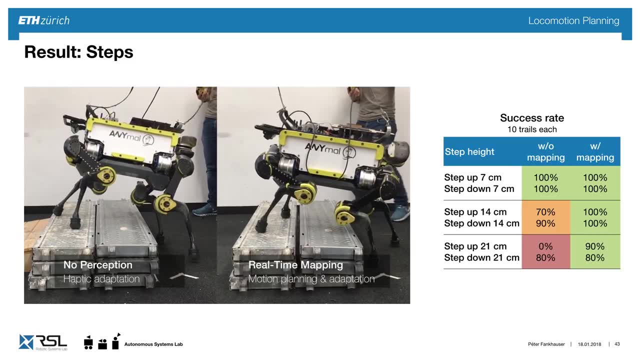 you see, with active mapping, the robot steps steps much more certain onto the obstacles And this actually takes the same step length but it's faster in the execution of the motion, And we have shown that we can achieve running over obstacles with up to a 50% of the leg length. 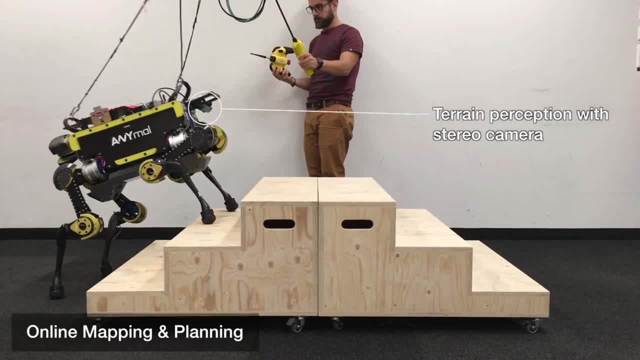 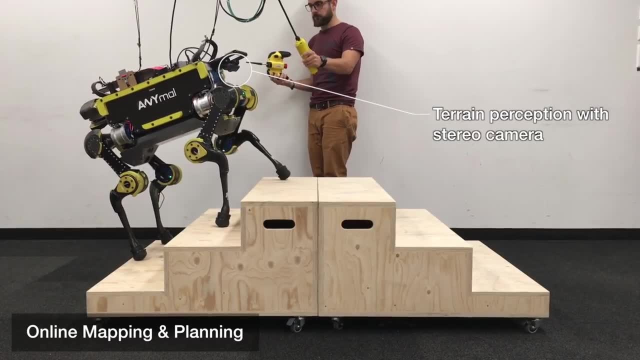 Now, in a little bit more complex scenario. we see here the robot walking over stairs, but we don't tell the robot that these are stairs. This is just an arbitrary terrain for the robot. We use the stereo camera in front of the robot. 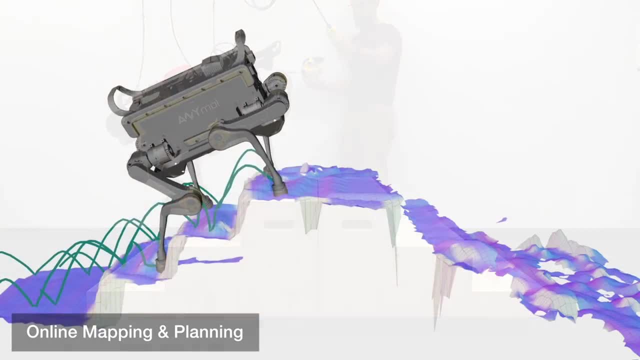 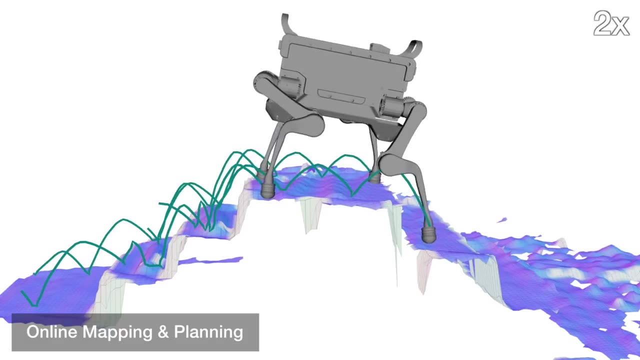 in order to create this elevation map And you see, in blue are the areas which are valid to step on and white ones the ones which are not. We clearly see that the map is not perfect. However, our framework can robustly track this motion. 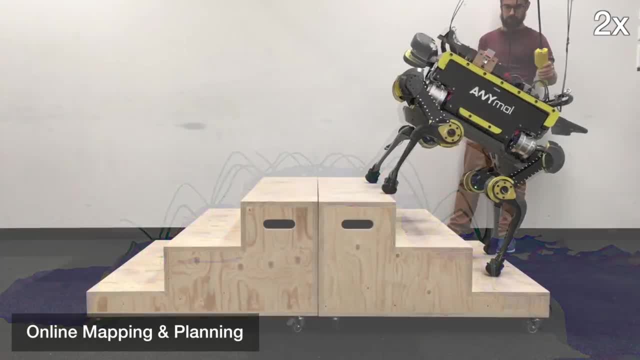 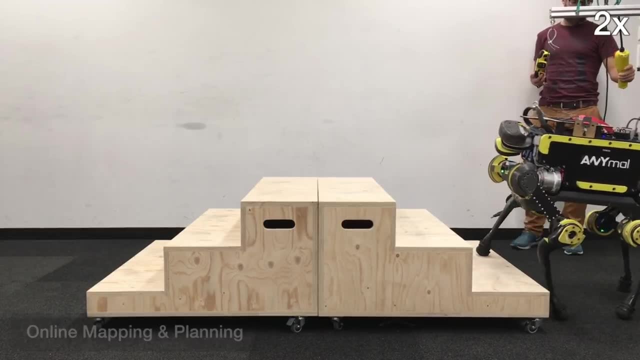 We're gonna see in a second how the hind legs slip. but due to our replanning process, this is not a problem and the replanning just continues from where it started. Since we have knowledge of the surface normals, we can feed that back to the controller. 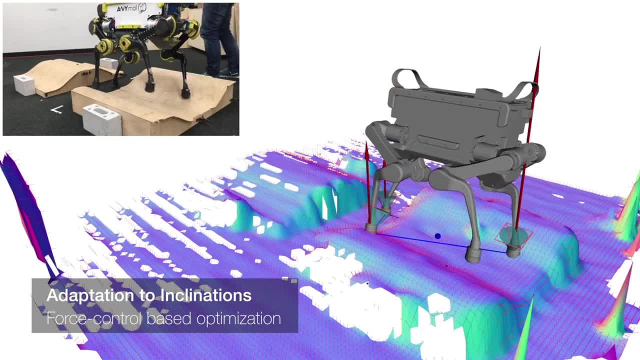 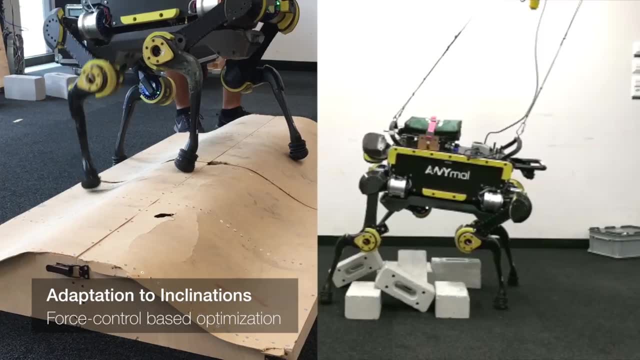 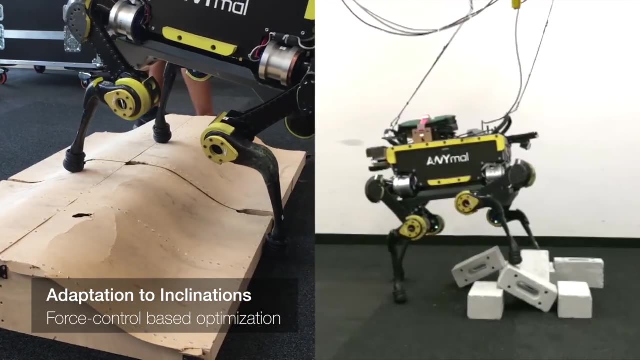 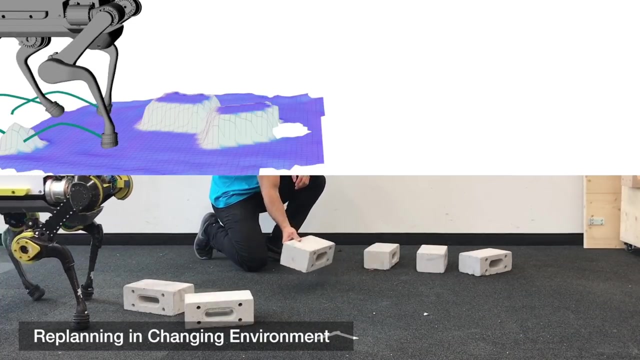 and use the force controllability of our robot in order to constrain our reaction forces on the ground, such as the robot does not slip on inclined surfaces like these. The reactiveness of our approach is shown here, where we throw stones in front of it. 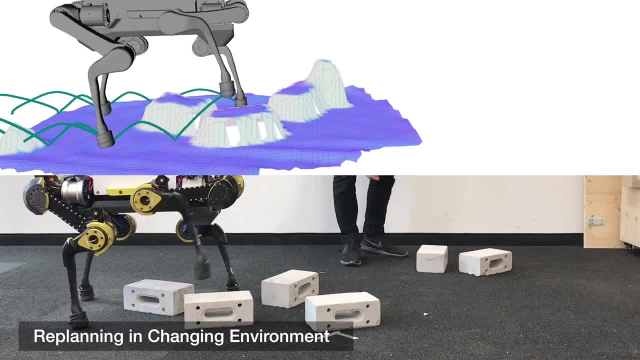 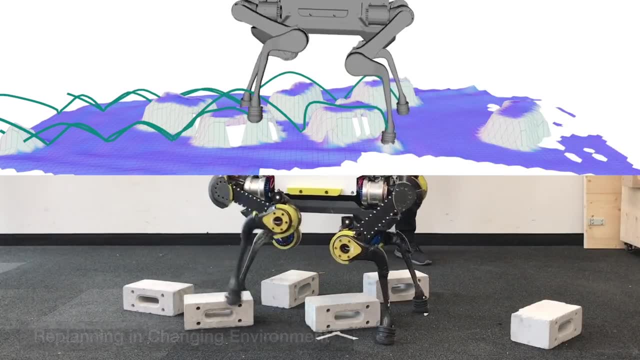 And we see in the map up there how quickly the entire process reacts and, since the replanning happens, it can walk safely over these obstacles that have been thrown in front of it. Here we show the robustness by pushing and pulling the robot. 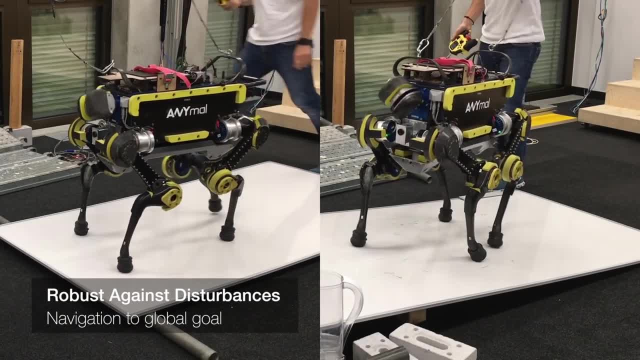 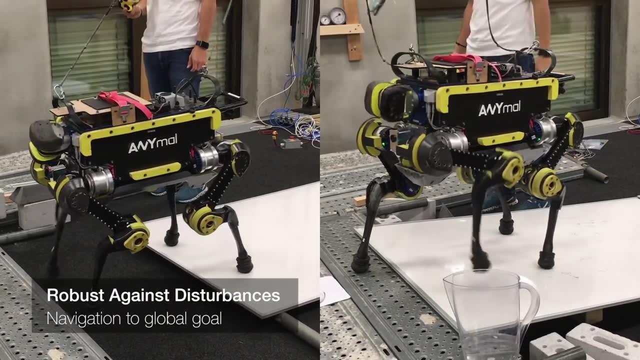 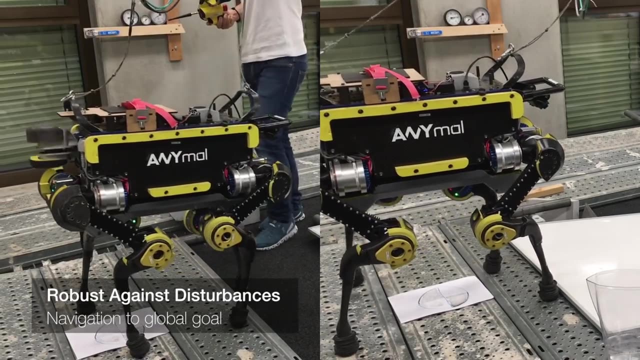 or changing the plate where it's standing on. And here it uses localization in order to navigate to a global goal in the room And, although we strongly disturbed it, the robot- the robot finds- generates the sequence to the goal location. And finally, this is to showcase the robustness. 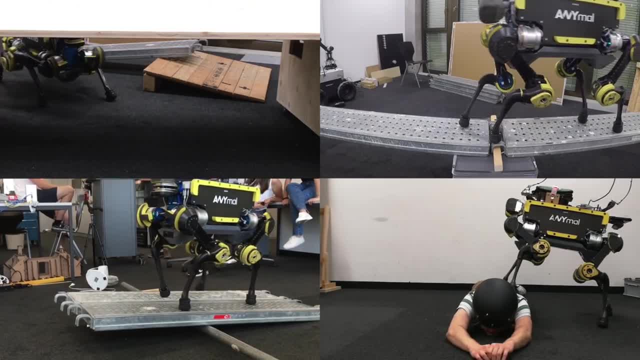 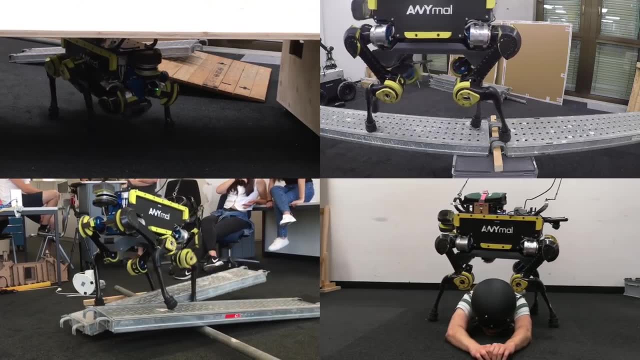 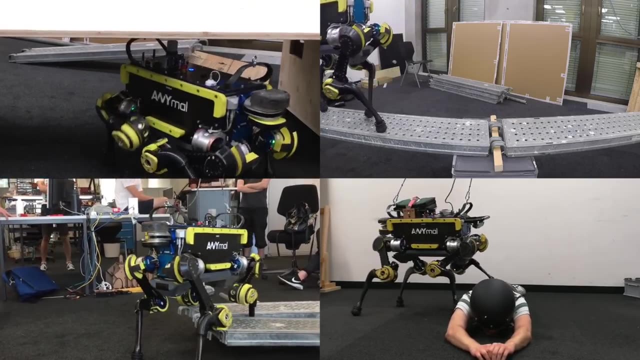 of the approach where we walk over moving obstacles, over a person, a soft body or even in a very narrow path. So this framework is really shown to be flexible in all of these environments and tasks. So now we have a robot walking over rough terrain. 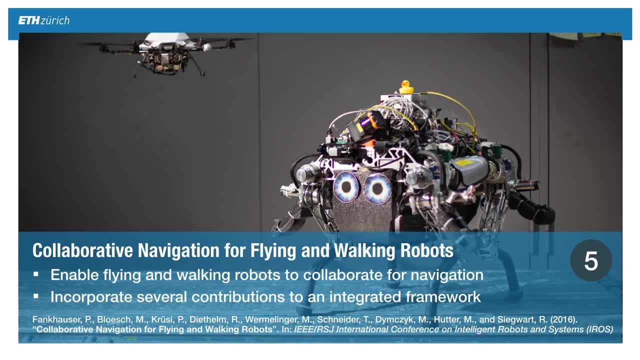 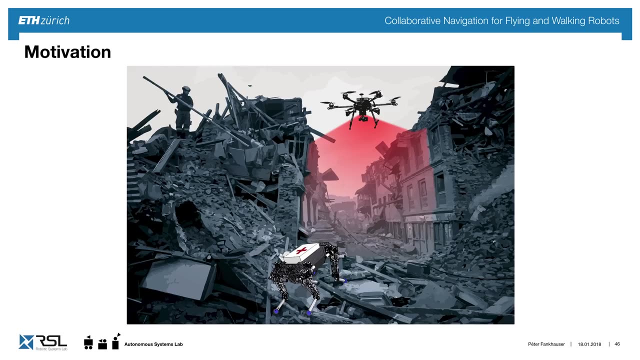 I want to expand a little bit and show how we did work the work with the collaborative navigation of a flying and a walking robot, And here it's about to use their different abilities to create a bigger framework. The motivation is that, from a flying viewpoint, 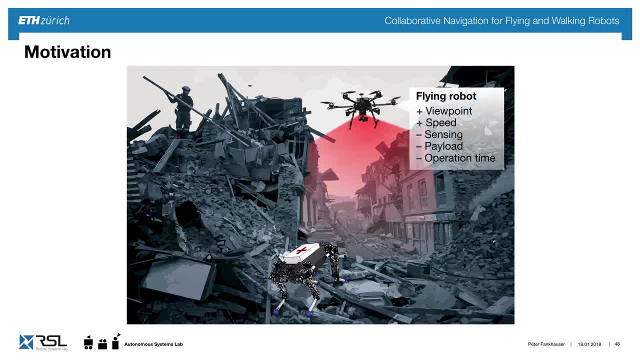 I can very quickly. the robot can see the terrain from up top and fly very fast around. However, it has limited sensing and payload capabilities and a limited operation time. On the other hand, I have a walking robot which has a rather low viewpoint. 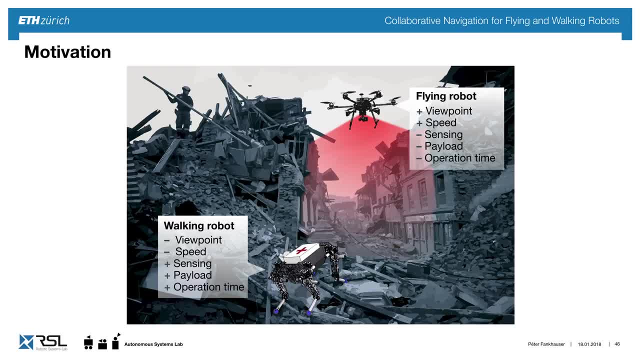 and is, compared to the flying vehicle, rather slow. However, it can carry high payload and sensing and has an operation time which is much higher than the flying vehicle. And this is the overview of the approach And I'm not going to go into the details. 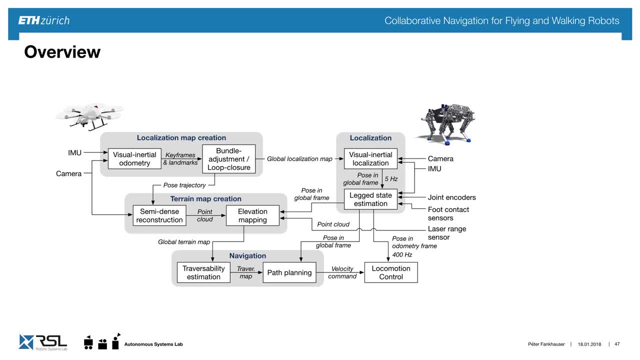 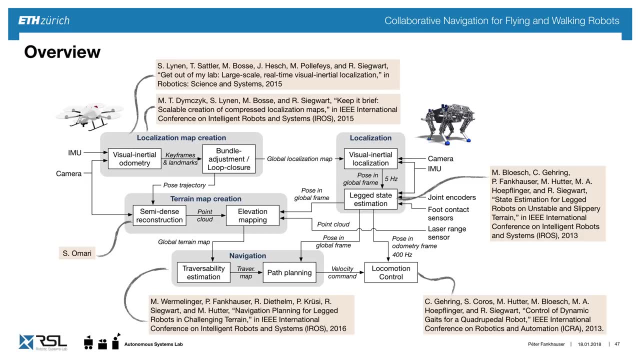 but I'd rather demonstrate the complexity that has gone into this work with many of my co-authors. So it's really all these technologies bringing them together, And I'm going to show you the demonstration that resulted from this work. So here the goal. 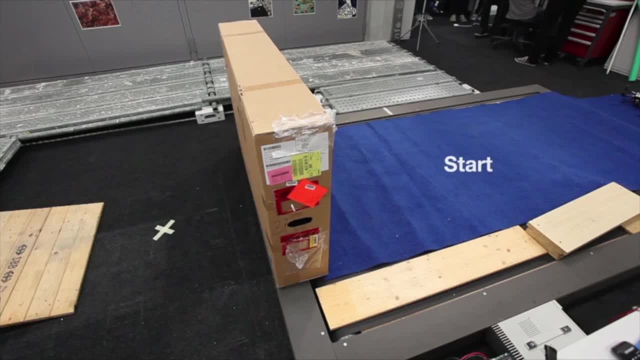 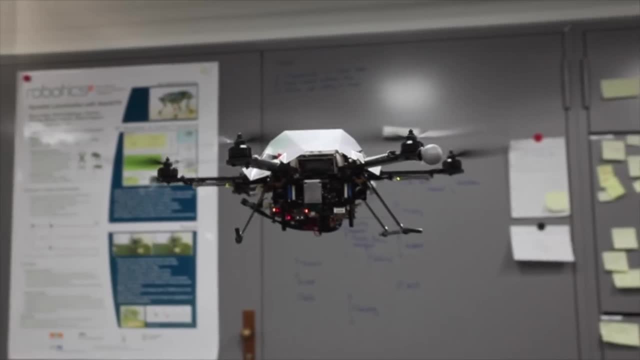 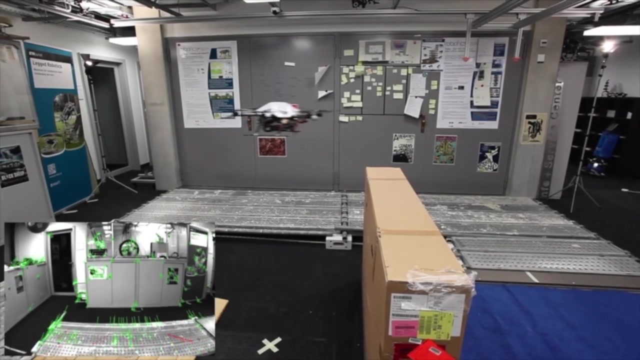 was to go from a start location to a target location where there's only one possible path and there's obstacles in between. So first we let the flying robot explore the environment And we see in the left bottom corner it creates a set of visual features. 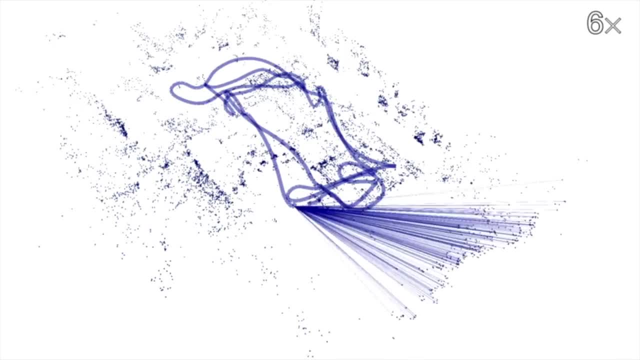 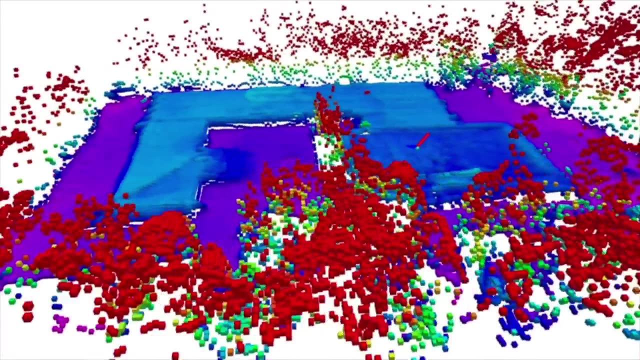 which are then added in a simultaneous localization and mapping framework to consistent map. We can use the camera images to create, with our elevation mapping framework, a dense representation of the entire field. So we can use the camera images to create, with our elevation mapping framework, a dense representation of the entire field. 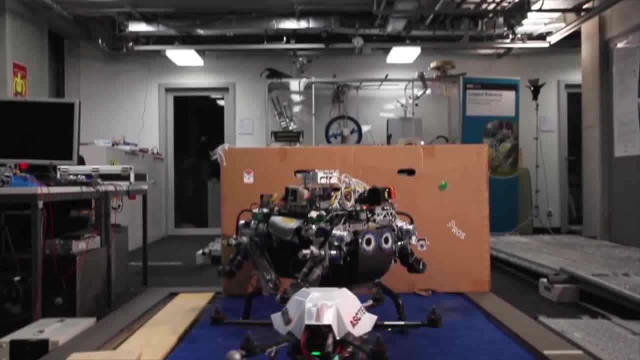 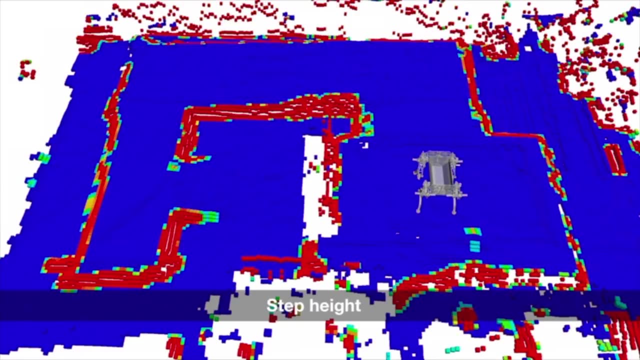 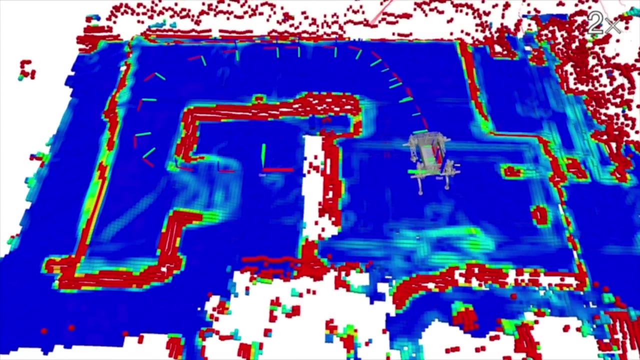 terrain, As these two maps are then transferred to the walking robot, which interprets them. So here: it looks at the traversability and then finds a global path from the start to the goal location And it starts tracking this, And while it goes, it uses another camera image. 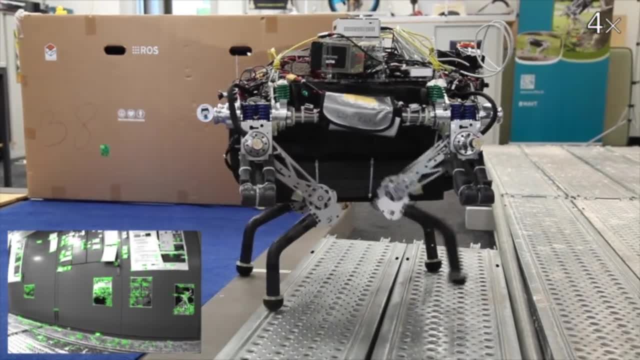 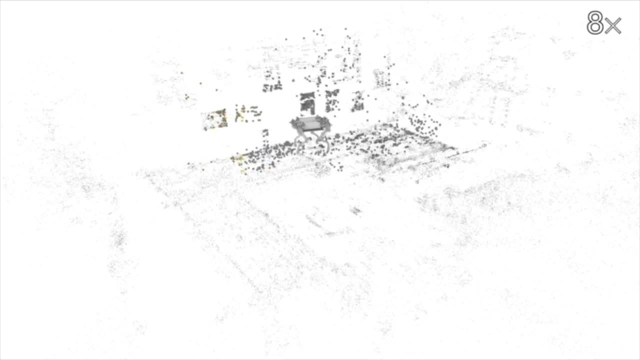 which is on the robot to localize itself within the map that was created by the flying vehicle. We can see here how it matches those visual features from the current viewpoint in the global map. It updates the map continuously and we are thrown an obstacle in front of it while walking. 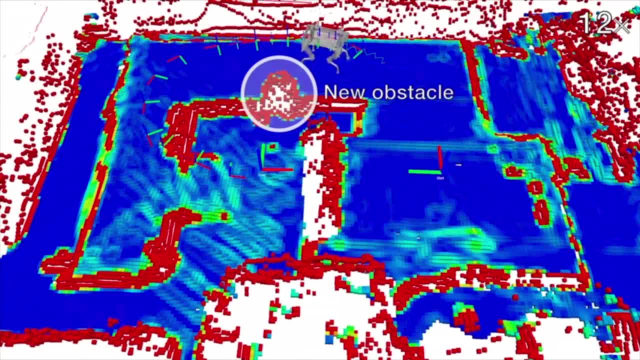 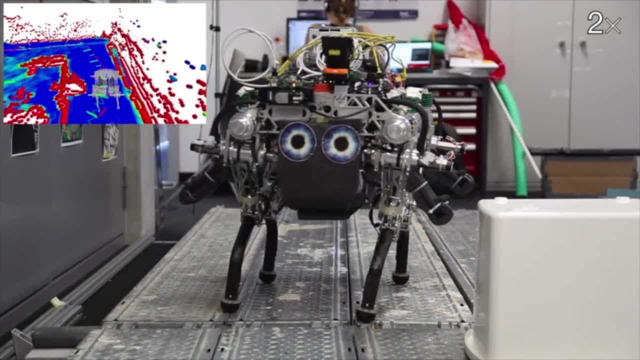 And since it updates, it replants the motion so that it can adapt to a changing environment and then make it safely from the start position, with help of the flying vehicle, to the goal location. With the help of the flying vehicle, to the goal location. 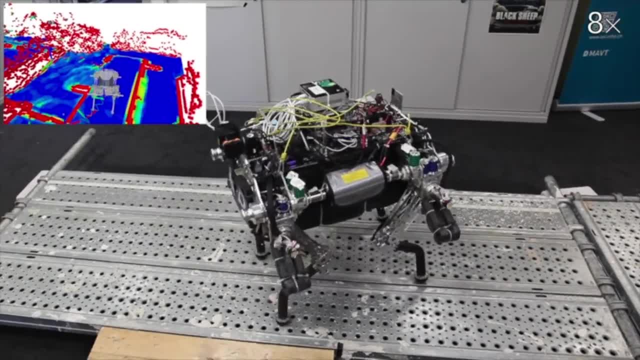 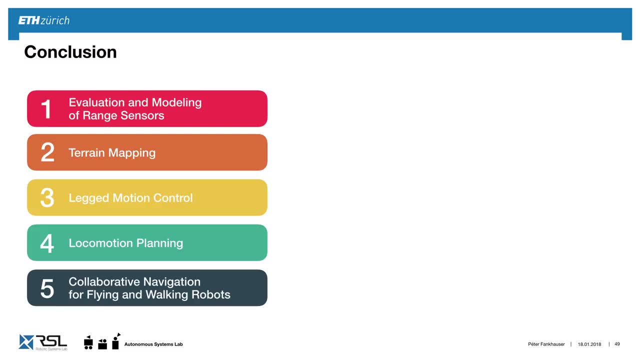 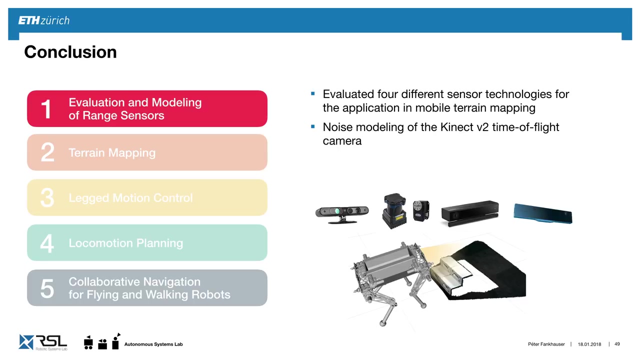 In conclusion, I have shown five contributions to the work in rough terrain locomotion with legged robots. First, I have evaluated different sensor technologies and showed them how they are applicable in mobile terrain mapping. I have modeled the noise for the Kinect version 2 time-of-flight camera, which is very important. 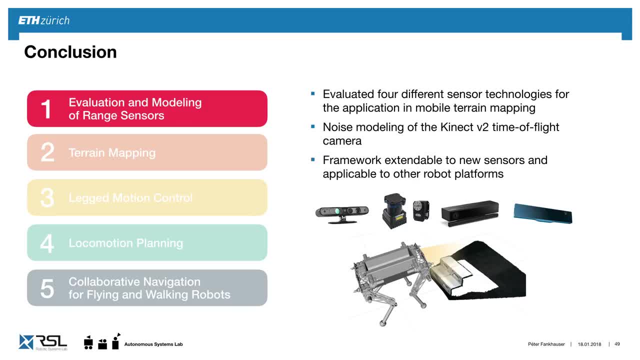 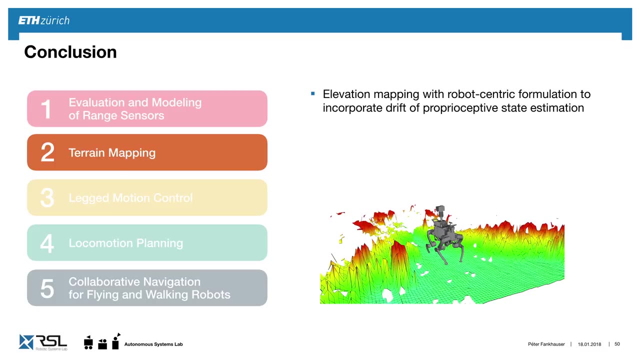 for mapping. This work can be extended as framework to new sensors as they are released, and our knowledge about the sensors is applicable to other mobile robots. In the second part, I have shown a robot-centric formulation of an elevation mapping framework which explicitly incorporates the drift of the state estimation. 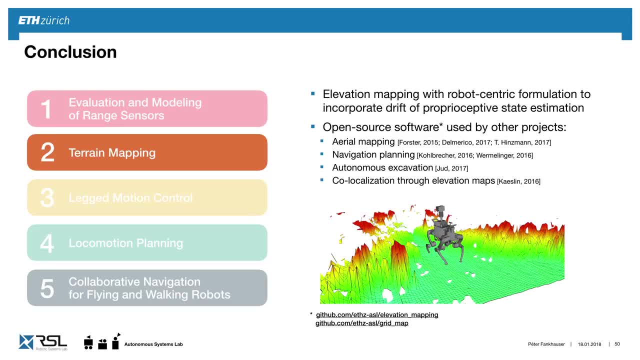 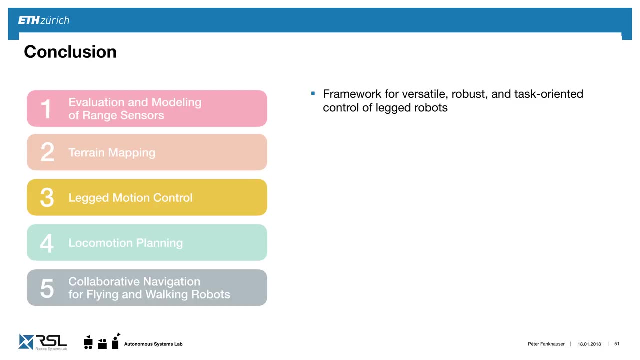 We have open-sourced the software, which has been used widely by many other projects, for example for aerial mapping, Navigation planning, autonomous excavation and co-localization. through these elevation maps For legged control, I have shown a framework for the versatile, robust and task-oriented 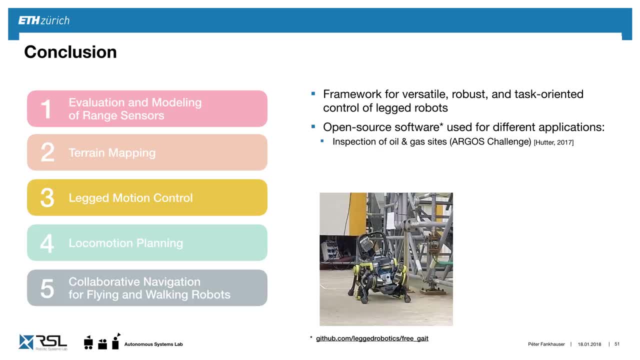 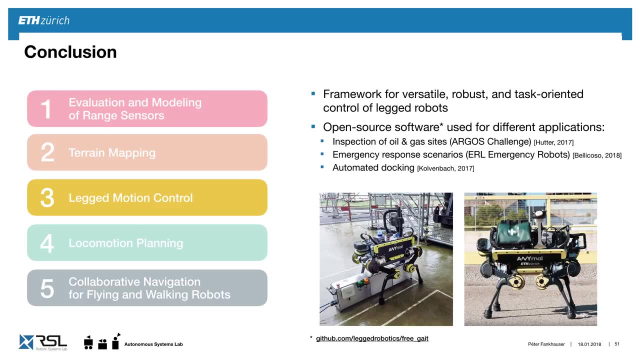 control of legged robots. Similarly, our software has been used in many applications, such as the Argos Challenge, the ERL Emergency Challenge, and we have created automated docking and even made the robot dance, where it listens to music and creates dance generation based on the sound of the